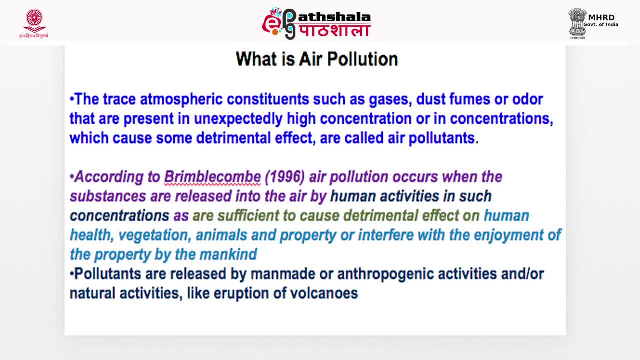 I have taken this definition from a celebrated atmospheric chemist, Peter Brimblecombe. He has been the editor of his prestigious journal Atmospheric Environment for several years. According to him, air pollution occurs when the substances are released into the air. 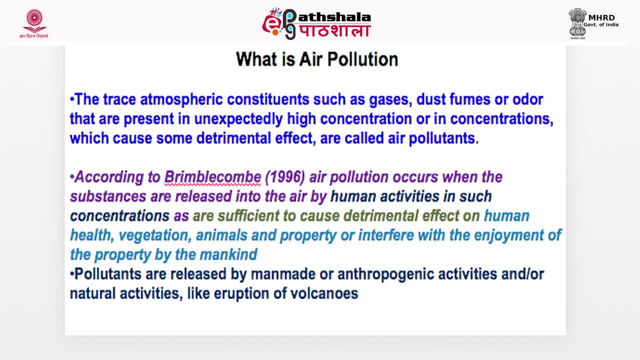 Substances that are pollutants. the substances which can cause harm are released into the air by human activities. Human activities, they are also called as anthropogenic activities or man-made activities- Such concentrations as are sufficient to cause detrimental effect. Now point is this: 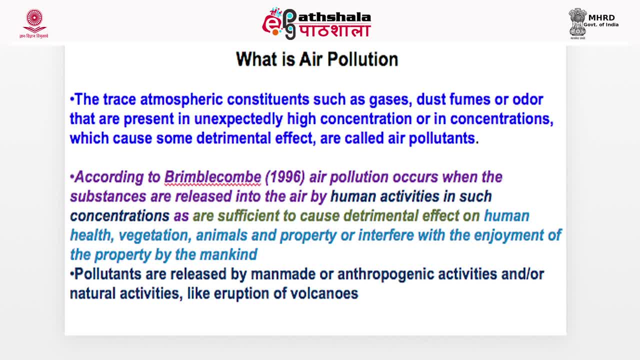 in such concentrations as are sufficient. If the concentration is less than sufficient to cause air detrimental effect, or it is so small that it doesn't cause any detrimental effect, then there will be no air pollution. So I repeat it: Air pollution occurs when. 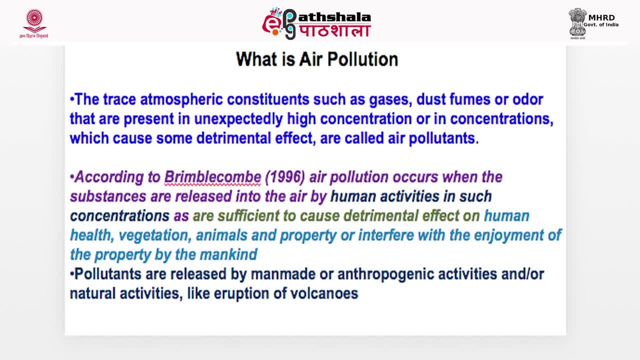 the substances are released into the air by human activities in such concentrations as are sufficient to cause detrimental effect on human health. The nature of the air pollution, which is the main measurement, is also some of the main reports for damage of air pollution in air pollution affected countries. 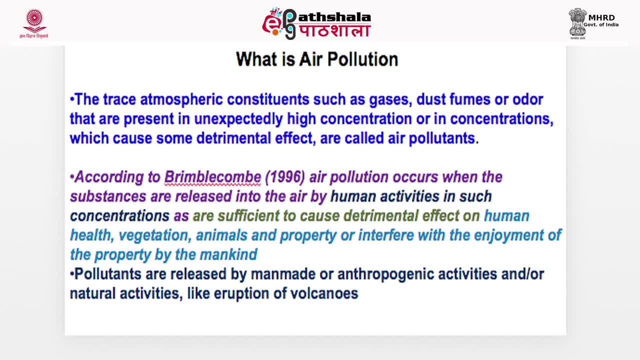 Every year, the radio frequency is released into the air and, due to these reports, the air pollution in the field is reduced by 2 to 3 percent. We have to remember the environmental impact of air pollution on many, many people, and this is a very important point. 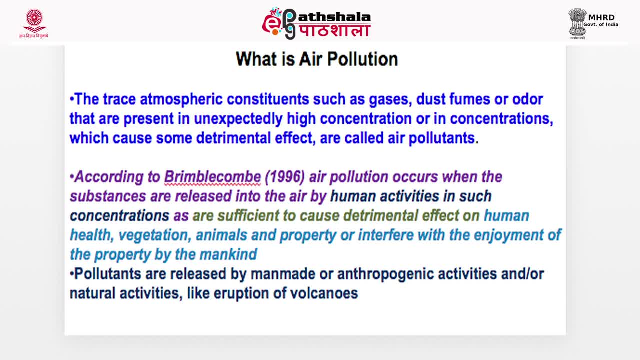 The air pollution is the cause of the air pollution and it is also the cause of the. Now one point is important: What is sufficient? There are pollutants like sulphur dioxide, this carbon monoxide ozone. they are present. Remember the concentrations of different. 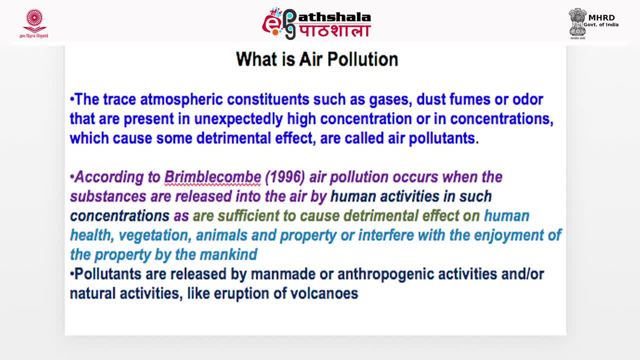 pollutants required to cause damaging effect are different, not they are same. So each compound has a threshold, an optimum limit. If the concentration exceeds that, only then it is a pollutant. Otherwise it is not a pollutant. So remember, everything can be. 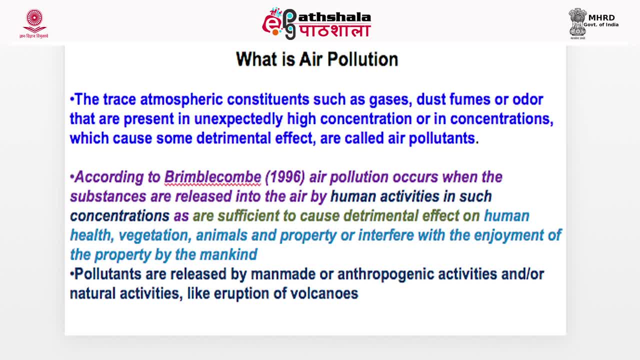 polluted, cannot be polluted, depending upon its threshold or limiting value. Otherwise, in an atmosphere, everything that you can see, which is toxic, which is harmful, it is present in the atmosphere. it is not damaging us because its concentration is small or below. 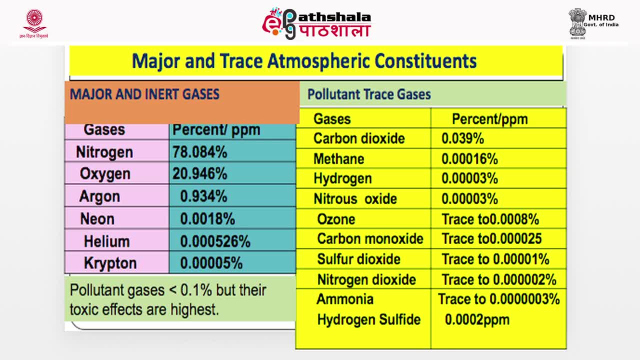 the threshold limit. Major trace atmospheric constraints are these: The major and inert gases are nitrogen, oxygen, argon, neon, helium and gas. The pollutant gases are less than 0.1%, but their toxic effects are highest, And these: 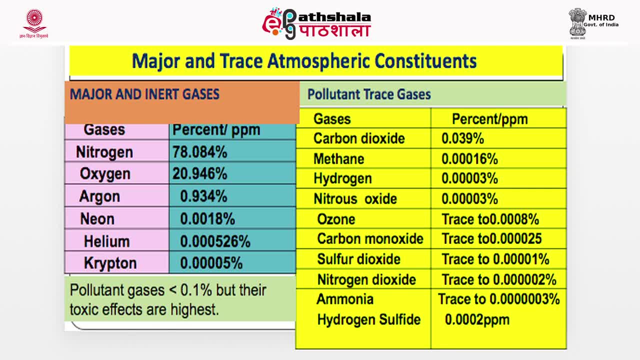 are pollutant gases. carbon dioxide- Remember carbon dioxide as such is not a pollutant, but it is involved in global warming, in increasing the temperature. That's why it is harmful. Methane, hydrogen, nitrous oxide, ozone, carbon monoxide, sulphur dioxide, nitrogen oxide. 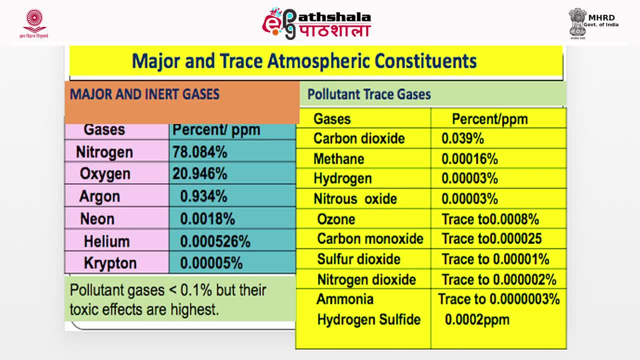 ammonia, hydrogen. remember, they are present in very small amounts, But amounts are small, but they are more harmful, Most notorious. So when we talk of air pollution, we are concerned with these, not with these. So for causing toxic effect, it is not necessary that something must be present in huge amount. 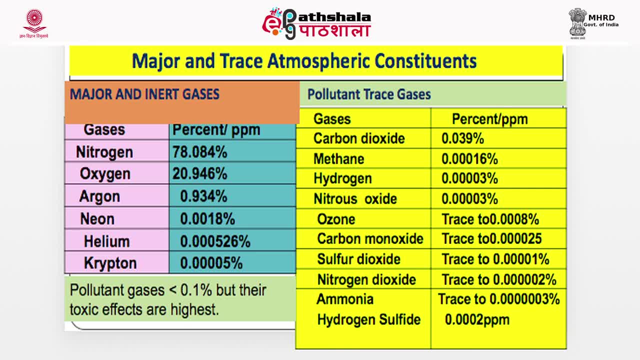 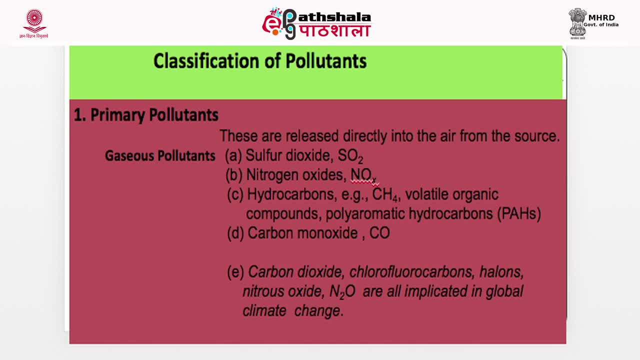 Not necessary. Even a small amount can be toxic, harmful, damaging, as in case of air pollutants. How the pollutants are classified: There are several kinds of classifications. First, I deal with primary pollutants, Those substances which are directly released into the air. 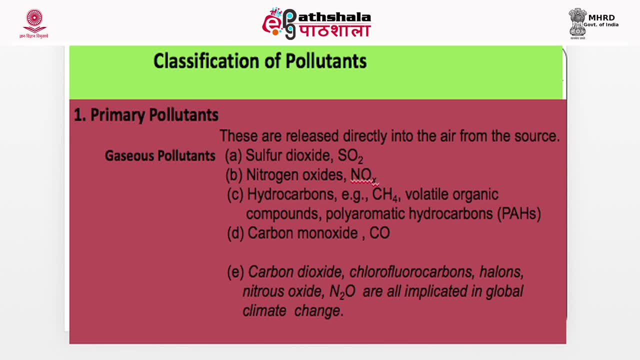 from the source are called primary pollutants. For example, when we burn coal, Coal has inherently sulphur present in it. When combustion takes place, along with carbon, sulphur also undergoes combustion. It is oxidized by sulphur and sulphur dioxide is released. 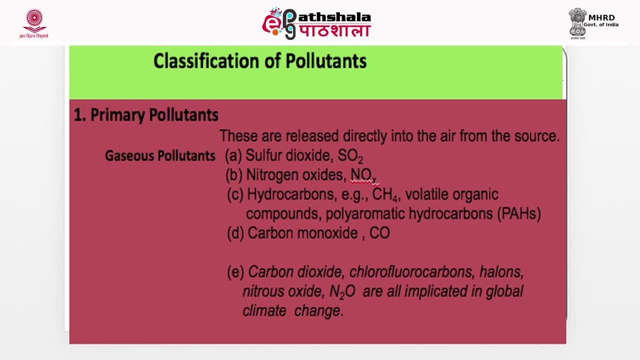 So it is directly released into the atmosphere, So it is a primary pollutant. Nitrogen oxide it is a, so they are all primary pollutants: Carbon dioxide, chlorofluorocarbons, Halons, nitrous oxide- and two are implicated in global warming, So they are all gaseous primary pollutants. 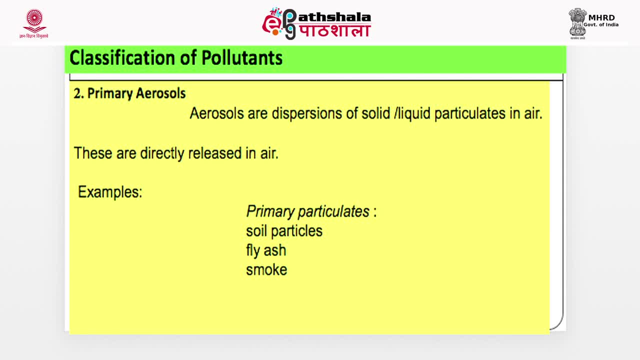 Next: aerosol: primary pollutants. Primary aerosol: what is aerosol? Aerosols are dispersals of solid or liquid particulates in air. Here is the dispersal medium: Solid particles or liquid drops. if they are suspended in air, then it is called a aerosol. 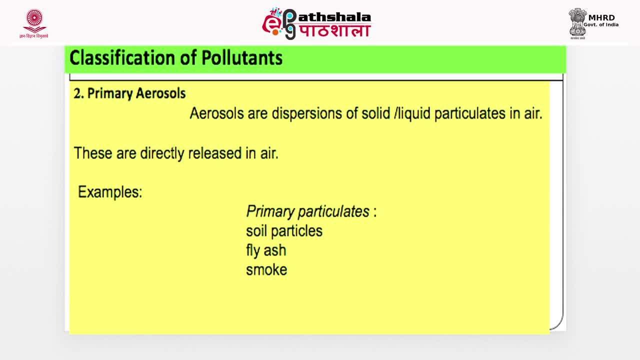 For example fog mist. they are aerosols. In both cases, the liquid drops are suspended in air. Primary aerosols are directly released in atmosphere, For example soil particles, fly ash, smoke. They are examples of the primary aerosols. Fly ash is formed. 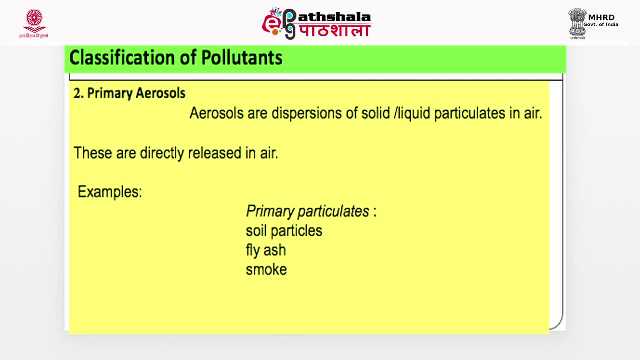 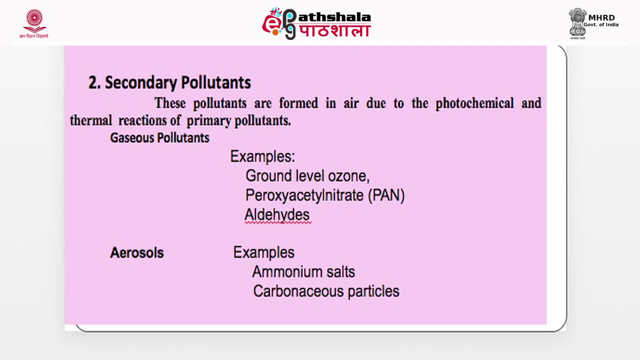 When the combustion in the power plant takes place, the fly ash is also released, Soil particles when any agricultural practice is done, when you work on the soil surface, the dust goes in the air smoke. there are primary aerosols, Secondary pollutants. Secondary pollutants: they are not directly released into the air. 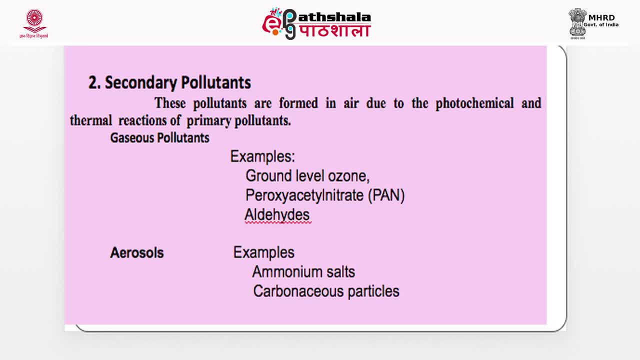 but due to photochemical or thermal reactions of primary pollutants among themselves. these are formed, So ground level ozone. How it is formed? It is formed by the reaction in atmosphere: Oxygen, atom and O2 gas, Peroxyacetal nitrate, photochemical smoke, aldehydes, by the oxidation of hydrocarbons, aerosols, ammonium salts. 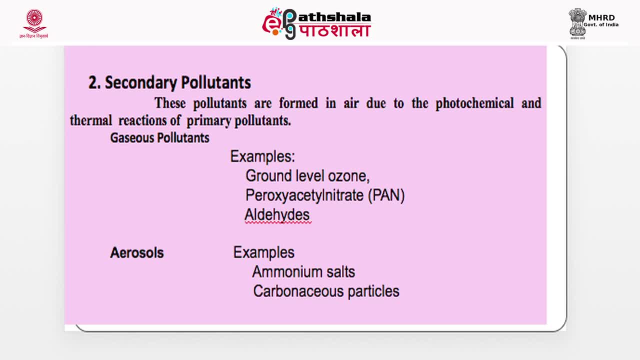 Ammonia and nitric acid. if they react, they form ammonium nitrate Ammonia. if it reacts with sulphuric acid, it forms ammonium sulphate. So they are aerosols, Carbonous particles, Particles, carbon particles. 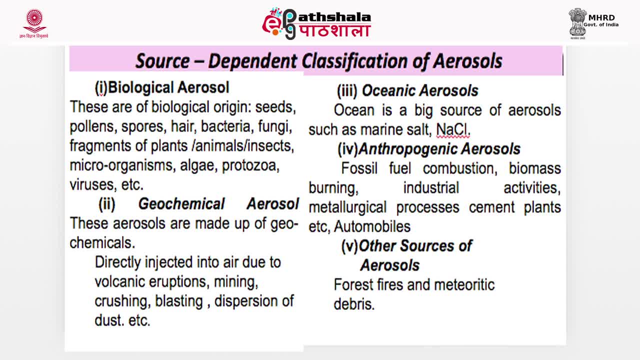 Source dependent classification of aerosols. This is the whether they are directly released in the atmosphere or they are not directly released in the atmosphere. Now, it is based on the source from where the aerosol has come. It is interesting to find out biological aerosols. 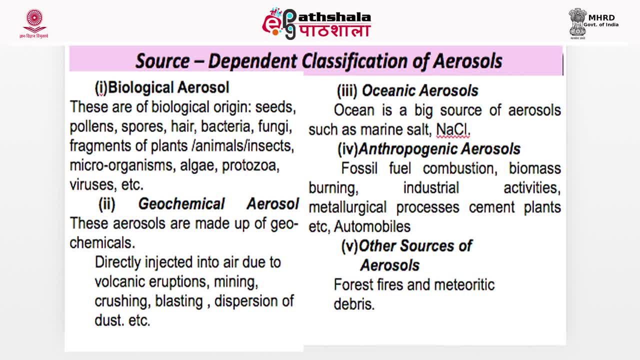 Seeds, pollens, spores, hair, bacteria, fungi, fragments of plants, animals, insects, Insects, microorganisms, algae, protozoa, viruses. they are all biological aerosols. They are suspended in air, Geochemical aerosols, That is. geo means earth. 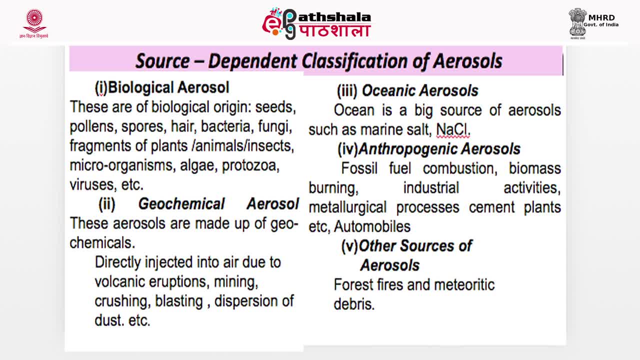 The chemicals taken directly from the earth. For example, when mining is done, during mining practice, some ore particles or other dust particles, they go into the atmosphere. Volcanic eruptions: this comes from the mother earth. The volcano releases lot of material. 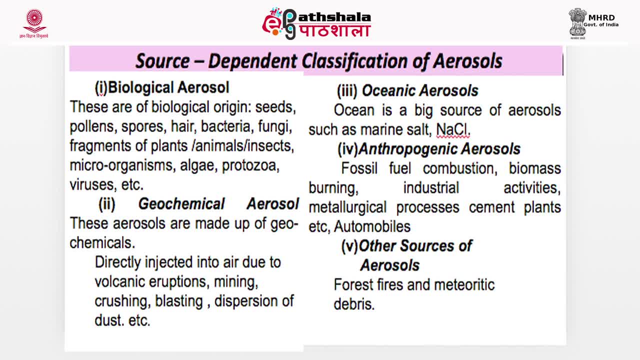 Sulfur dioxide, dust particles, chemicals- okay, Oceanic aerosols. Ocean Ocean is a big source of aerosols, particularly sodium chloride or marine salt, And this air it releases into the air Anthropogenic aerosols, man-made. 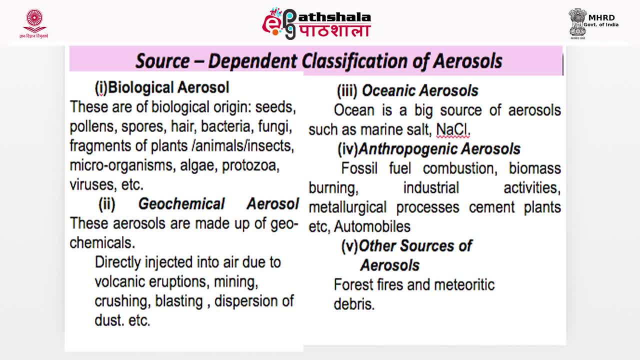 For example, if coal is undergoes combustion, then shoot particles. The smoke comes out, it gets particles. Industrial activities: Whenever the metallurgic iron is made copper is made cement, is made atomoids, they all release particles in the atmosphere. 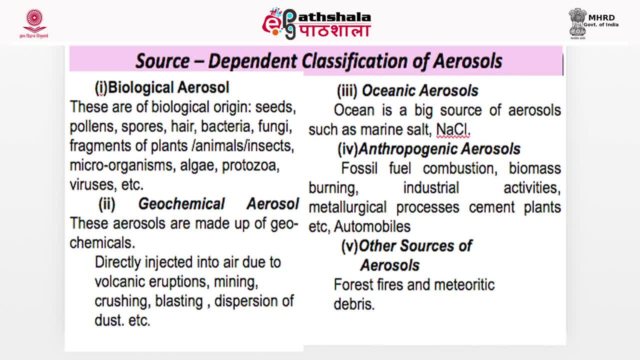 Other sources of aerosols are forest fires, ambient kinetic debris. You must have heard. recently there was a fire here in our country and elsewhere. When the fire takes place in the forest, a large area undergoes combustion And then, due to the combustion of wood leaves, the particles are released. carbon particles are released. 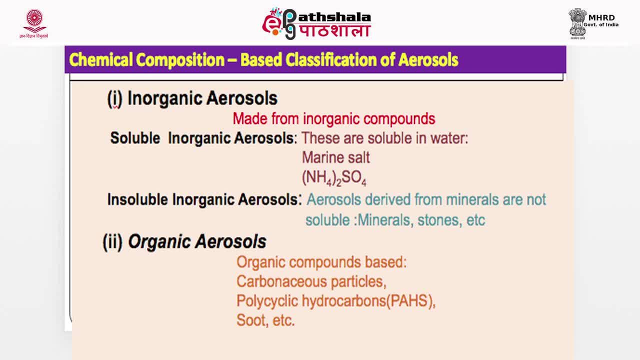 They cause aerosol formation. Chemical composition based classification, whether organic or inorganic. Those made from inorganic compounds are inorganic aerosols. These can be soluble or insoluble. two types, For example: ammonium sulphate. This is aerosol. 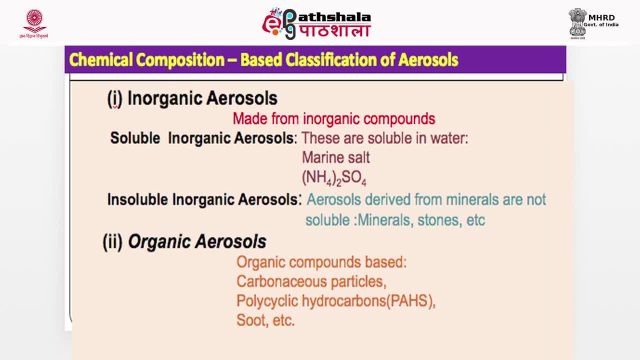 Marine salt, NaCl. They are soluble matter. They are inorganic but soluble. Insoluble minerals, stones. They are inorganic but they are not soluble. Organic aerosols basically made from organic compounds, From carbon Organic compounds, carbonous particles, polycyclic aromatic hydrocarbons, soot, etc. 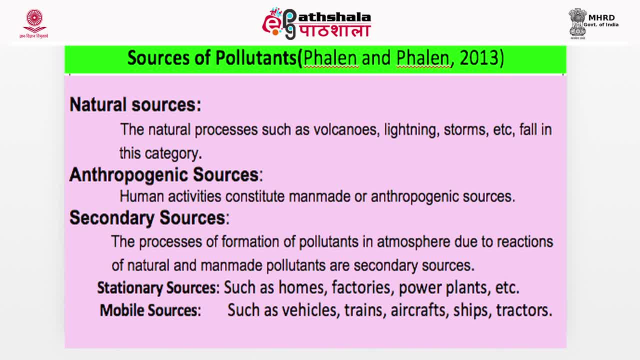 Sources of pollutants: Natural sources. The natural sources such as volcanoes, lightning, storm, etc. fall in this category. Lightning stones- Volcano is a big source of Dust particles. sulphur dioxide Lightning- big source of nitrogen oxides. 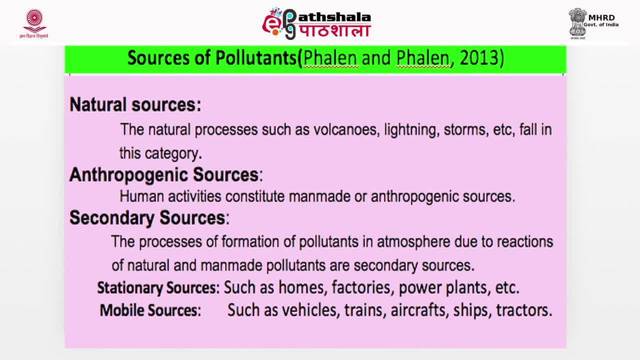 When lightning strikes, the temperature is very high. At that temperature nitrogen and oxygen combine for nitrogen oxides, So it is a big source of nitrogen oxide. pollutants, Storms, Anthropogenic sources, man-made sources, Human activities- There are all kinds of activities. 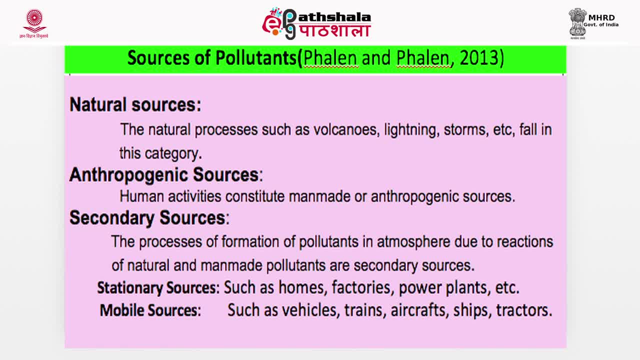 There are several kinds of activities, starting from cooking at homes to running factories. Secondary sources: The process of formation of pollutants and atmosphere due to reactions of natural and man-made pollutants are secondary sources, For example, stationary sources. These are of two types. 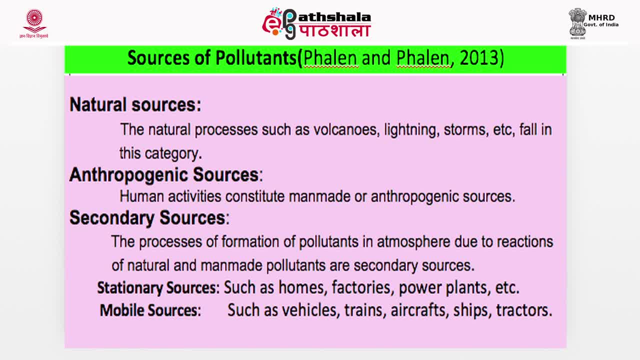 Stationary that is stable, They do not move. Remember Homes, Homes. they have kitchen Factories, power plants. they do not have legs, They do not move, They remain a standard workplace. They are stationary, Mobile sources. 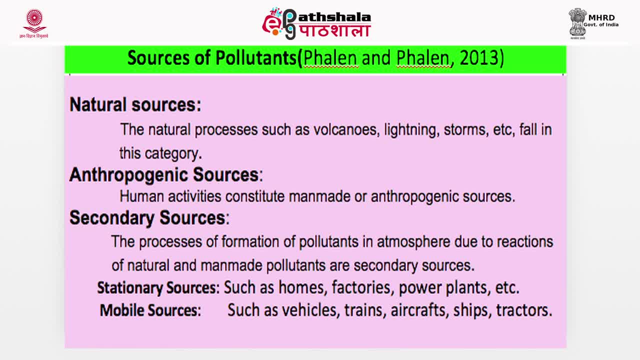 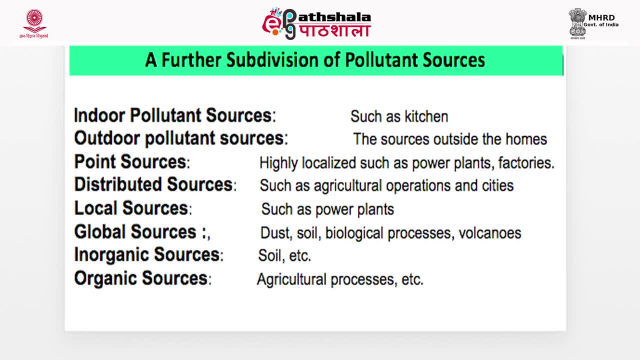 For example, vacuums, Trains, aircraft, ships. They are stationary, They are source of pollution, But these sources are mobile sources. A further subdivision of pollutant sources: Indoor pollutant, Such as kitchen. Outdoor pollutant sources, such as, which are outside the homes. 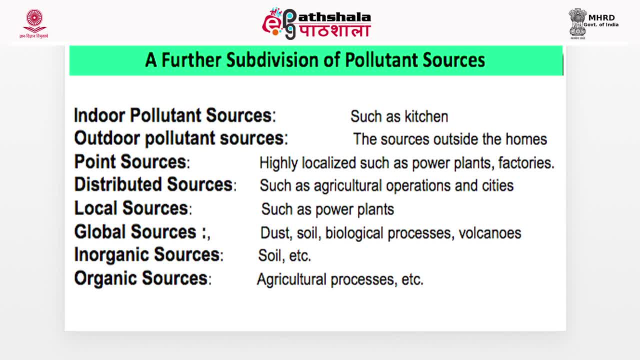 Anything which is outside the home gives pollution. Point sources, Highly localized. There is a power plant, factory, Power plant is one point. There is no power point in the vicinity. Distributed sources, Agriculture operations, Fields, One field, Another field. 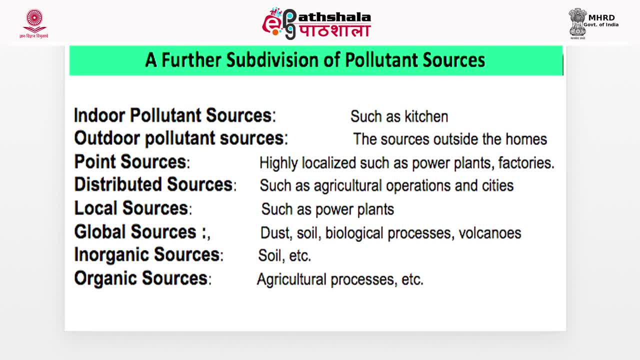 Another field, One city, Another city. They are distributed sources: Local sources as power plants. Global, Which are globally concerned, Biological processes, Volcanoes. They can affect several countries. Inorganic sources as soils. Organic sources as agriculture processes. 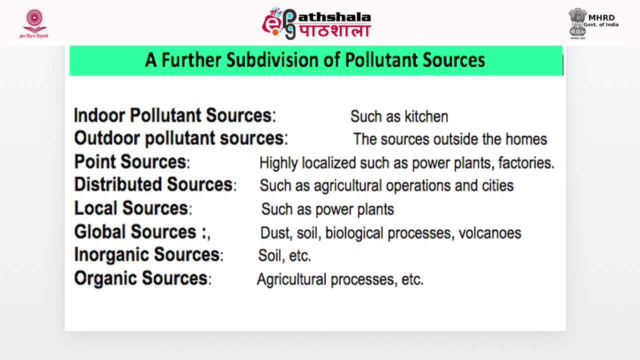 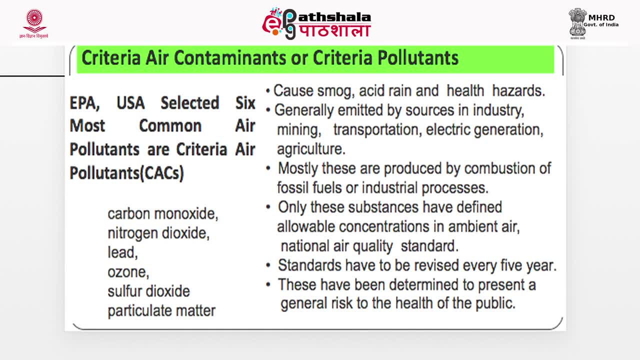 So actually there are numerous types of classification you will find in literature. These are some of which I discussed here: Criteria, here Contaminants, or criteria pollutants. Environmental Protection Agency of USA selected six most common here pollutants, which is called criteria pollutants. 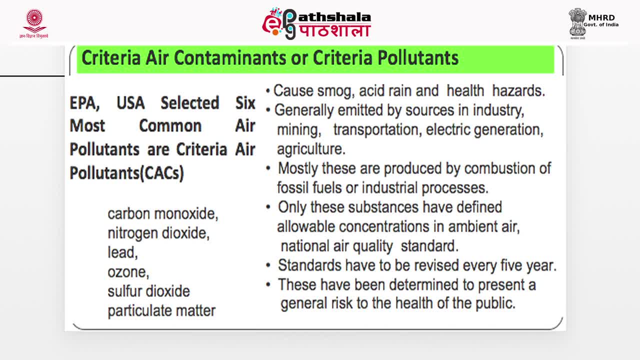 They are carbon monoxide, nitrogen dioxide, NO2, lead- that is, metal ozone- O3, sulfur dioxide and particulate matter. These Criteria here Contaminants or CAC, they are called What they do, They cause smoke formation, acid rain and health hazards. 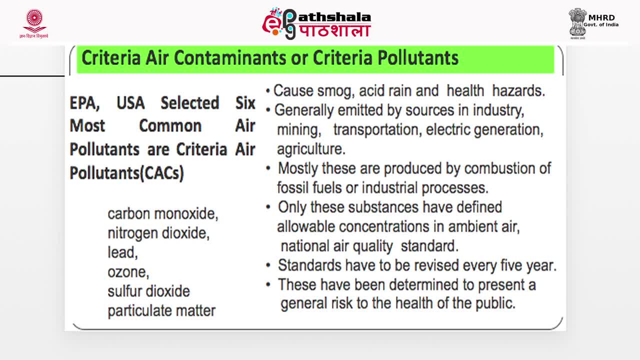 Generally emitted by sources in industry: Mining, transportation, that is, movement of vehicles, electric generation, agriculture. Mostly, these are produced by combustion of fossil fuels or industrial. What is fossil fuel? A fuel which is taken out from the mother earth. The earth is the source. 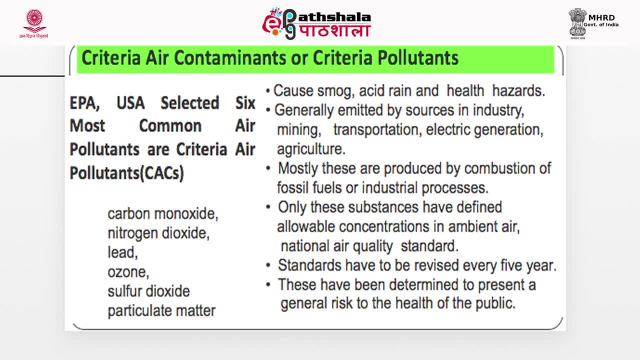 For example coal, For example petroleum, For example diesel, For example natural gas. They are all fossil fuels. Only these substances have defined available allowable concentrations in ambient air and national air quality standards. For them, the standards have been designed. 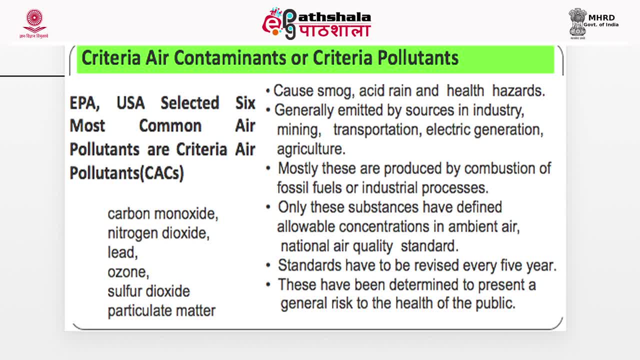 The soap no more than this much carbon or carbon monoxide in the atmosphere. A vacuum should not release more than this much amount of CO, this much amount of nitrogen oxide. That is why the pollution check is done on the vacuums. It is based on the amount that must be checked. 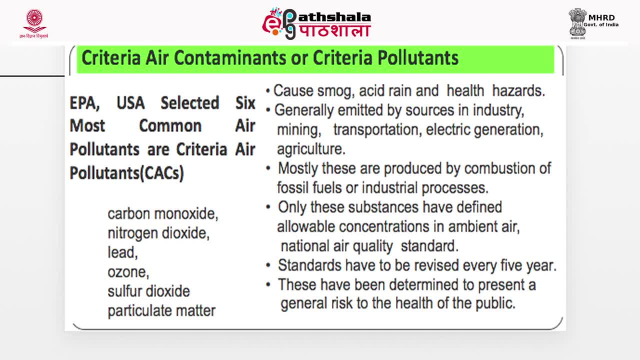 And this standard is revised every five years. These have been determined to present a general list to the health of public. Remember, In case of pollutants, you can never say what are the possible toxic effects of carbon monoxide, Because you know two toxic effects. it may have ten other which you do not know. 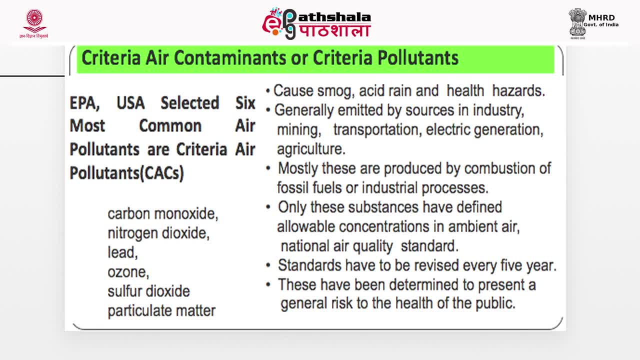 So you can give a general idea that this carbon monoxide can do this. So that is why these have been determined to present a general list to the health of the public. And this is the specific effect: Hazardous. This is another thing. 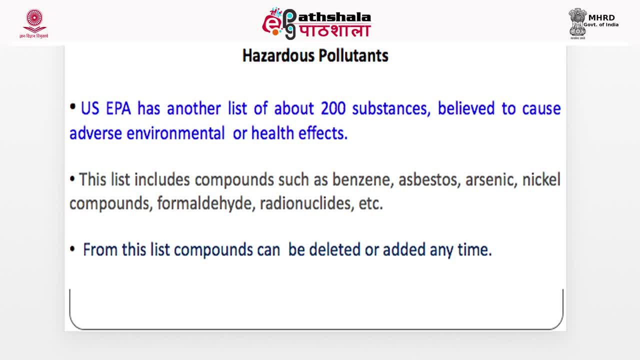 This is well known term. US Enmant Protection Agency has another list of about 200 substances believed to cause adverse environmental or health effects. Okay, And these include such well known compounds: benzene, asbestos, arsenic, nickel compounds, formaldehyde, radionuclides, etc. 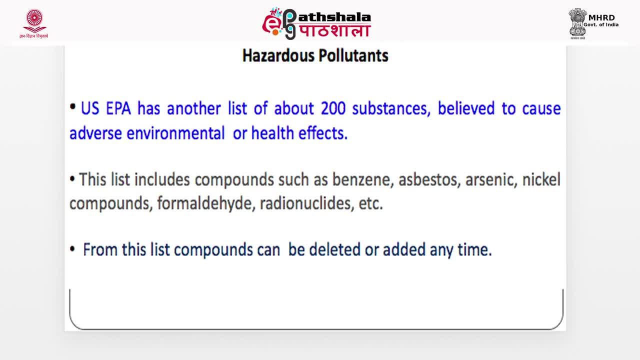 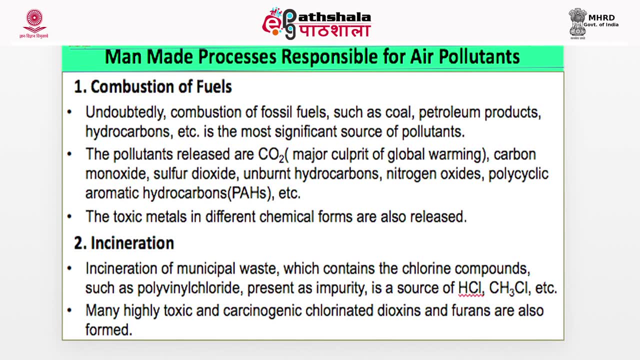 From this list. compounds can be deleted or added any time, Right, So this is always under revision. Man-made processes responsible for air pollutants. How we are most important is combustion of humans. What is combustion? The oxidation of any substance by oxygen is combustion. 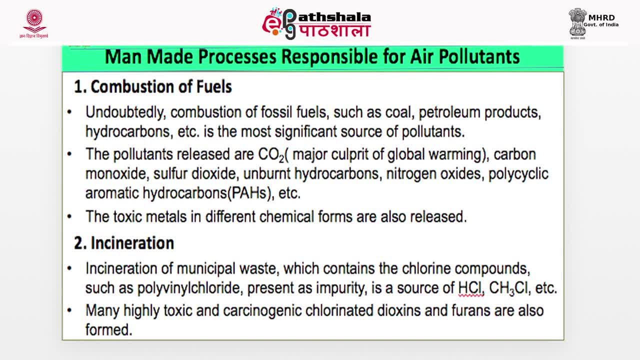 And why combustion is carried out by human beings? Because it gives energy, As energy is used for many things. Undoubtedly, combustion of fossil fuels such as coal, petroleum products, hydrocarbon, etc. Is the most significant source of pollutants. Pollutants released are CO2.. 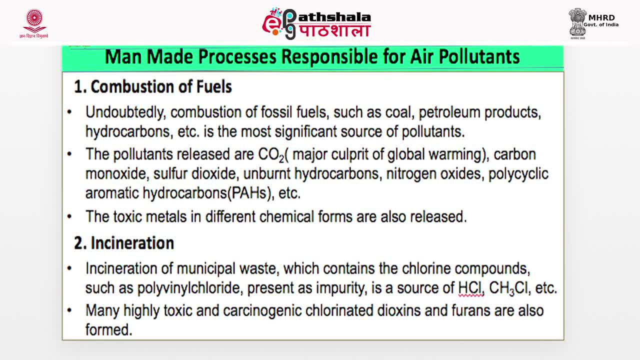 Major culprit of global warming: Carbon monoxide, sulfur dioxide, unburnt hydrocarbons, Nitrogen oxides, polycyclic aromatic hydrocarbons. This is- it has a symbol of PAHS- Unburnt hydrocarbons. 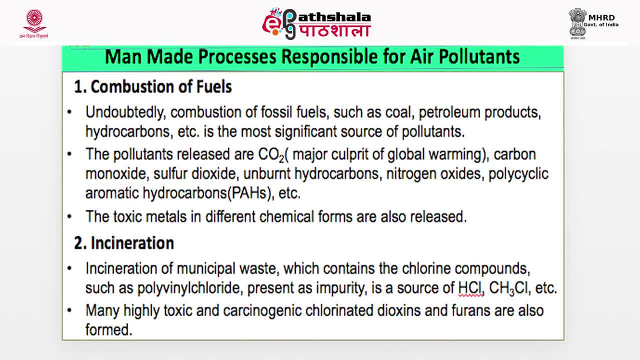 Remember your car, your scooter, your vacancy, The petrol or diesel. they are nothing but hydrocarbons. If the hydrocarbon That is not, Which has not gone undergone combustion And it is released to the atmosphere, That is unburnt, hydrocarbon has been released to the atmosphere. 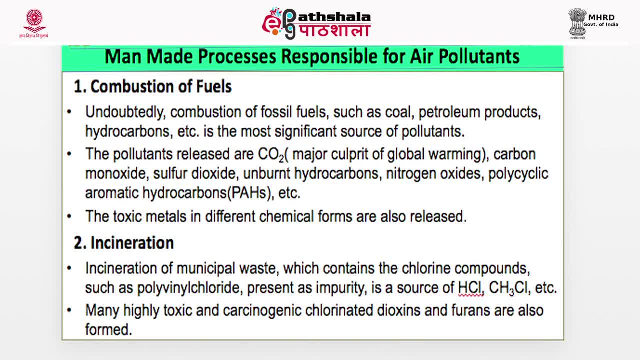 And pollution has been caused. The toxic metals in different chemical forms are also released by combustion. For example, if coal has some mercury, then mercury will also be released. Incineration: What happens? The municipal deaths in many times, In particularly in mahallas, in localities. 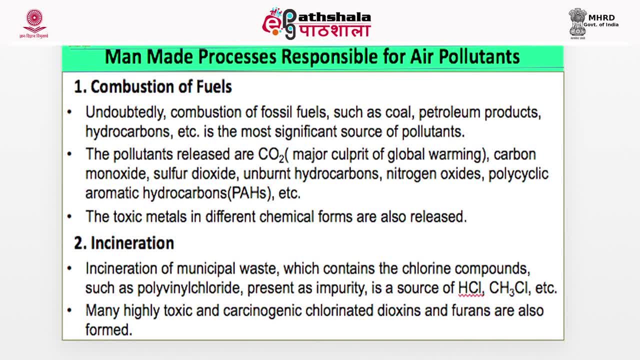 The sweeper comes and wards it, So it is a matchstick to it And it undergoes combustion. But it is a dangerous thing. It should not be done Because it has plastic material Which have chlorine compounds And these produce highly toxic, carcinogenic chlorinated dioxins and purines. 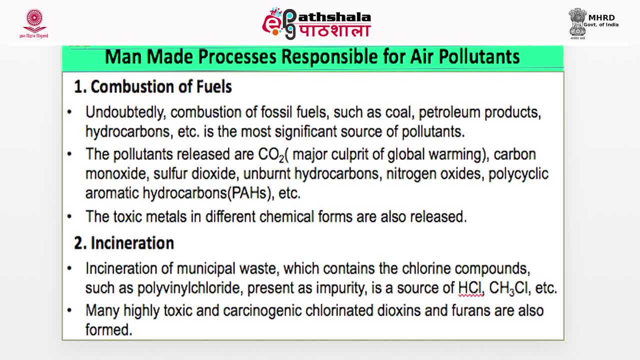 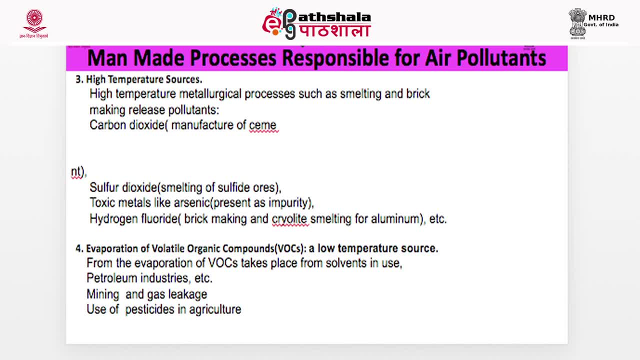 So that is why any plastic should not be allowed to undergo combustion. Manmade processes are responsible for air pollution. High temperature sources: These are the names of high temperature sources. High temperature metallurgical processes, Such as smelting of Smelting and brick making release pollutants. 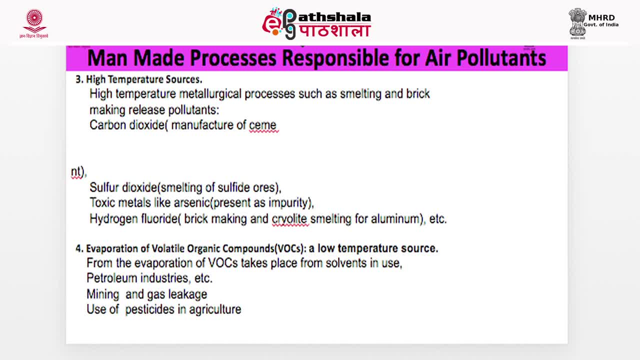 For example, if you see How the iron is made, The temperature is very high. It is red hot. I have seen The iron flowing When brick eat. Brick making releases pollutants: Carbon dioxide, manufacture of cement, Sulphur dioxide, smelting. 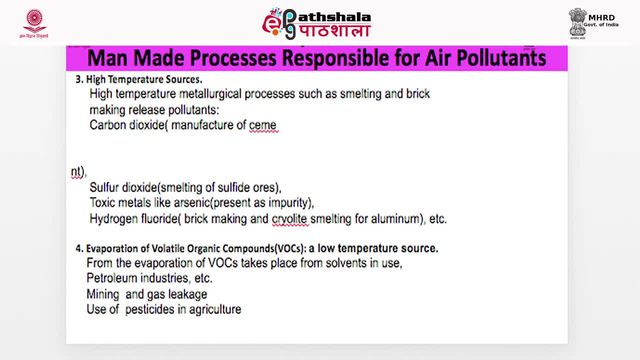 Sulphur dioxide smelting of sulphide ores. You use copper sulphide to form To get copper metal. Toxic metals like arsenic present as impurity. Hydrogen fluoride brick making Cryolite smelting for aluminium. They are source of hydrogen fluoride. 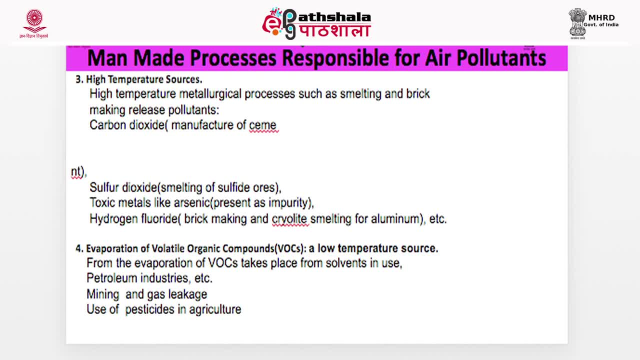 Evaporation of volatile organic compounds- VOCs. Now, VOCs is a Is a name. This is well known name. They are pollutants, Volatile organic compounds. which has room temperature They evaporate From. That is why they are called VOCs. 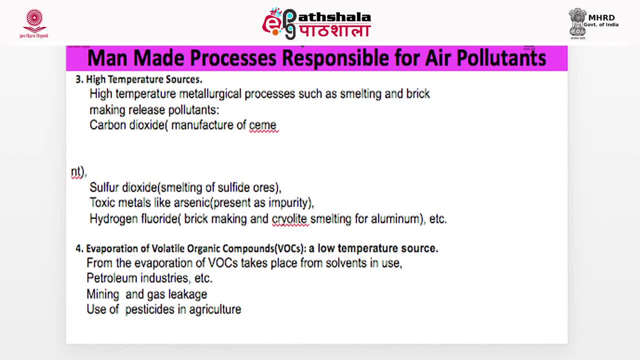 From the evaporation of VOCs Take place from solvents in use. Many kinds of solvents are used In industries. Solvents are used in Paints, Petroleum industries, Mining and gas leakage. Uses of pesticide in agriculture. So they are. 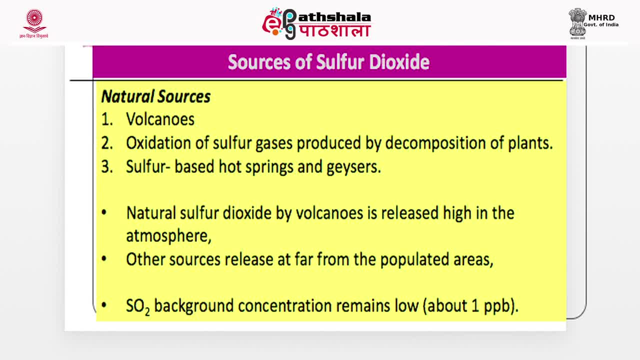 The sources of Volatile organic compounds. Sources of sulphur dioxide, One of the major pollutants, SO2.. The combustion of sulphur S plus O2 forms SO2.. The natural sources: Volcano- It comes once in a while. 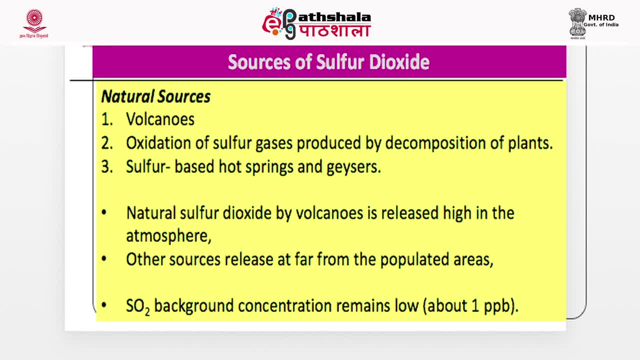 This is common thing: Oxidation of sulphur gases produced by decomposition of plants. But remember, plants have very small amount of sulphur, So Sulphur dioxide released by plants will not be much, But it is there, Sulphur based. 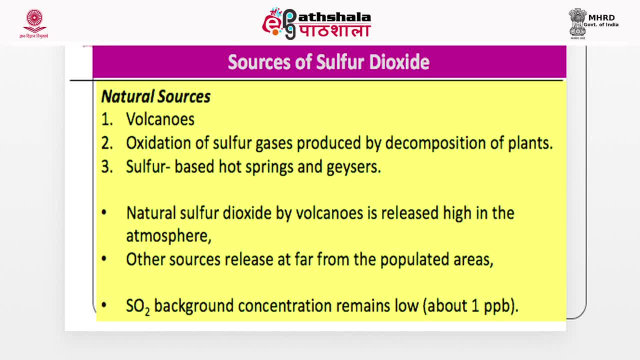 Hot springs And geysers. This is also not a big source Natural sulphur dioxide by volcanoes Released high in the atmosphere. Yes, Where there is a volcanic activity, At that place, Huge amount of sulphur dioxide May be released. 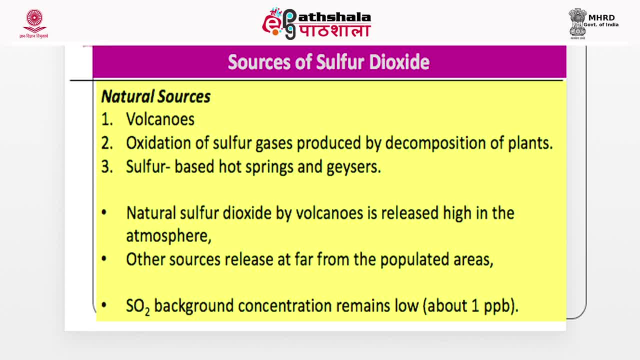 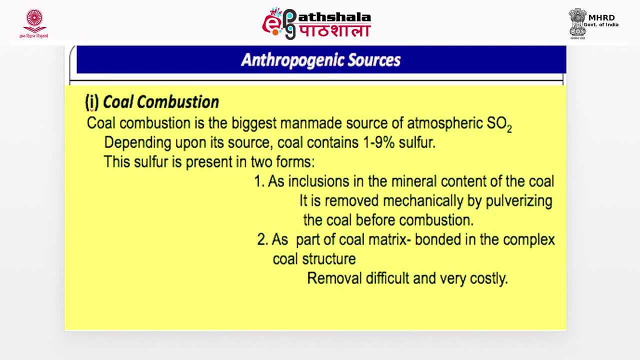 SO2 background concentration remains low, About one parts per billion At any time in the atmosphere. Normally, If it is not much polluted, This much Sulphur dioxide is always present. Manmade sources: Biggest source is coal combustion. Coal combustion is the biggest manmade source of atmospheric SO2.. 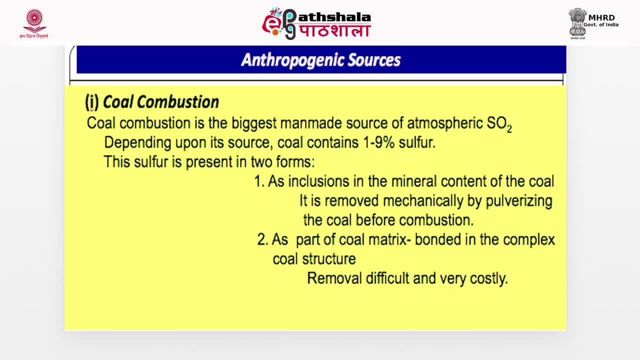 Depending upon its source. coal contains 1 to 9% sulphur. One is very low, 9% is very high. For example, Poor quality coal, Lignite. It has high sulphur In India, The sulphur. 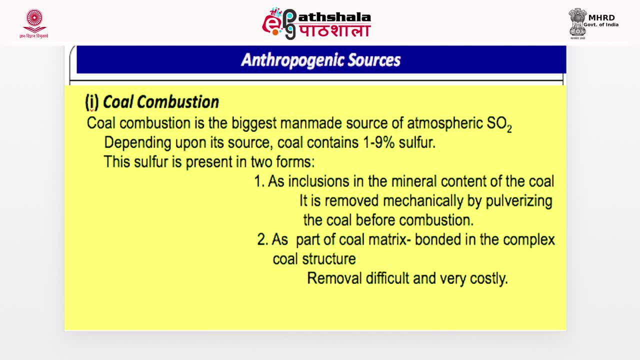 In coal is not much high. The sulphur is present to two forms in coal As inclusions In the mineral content of the coal Mineral, For example FeH2.. Some inorganic sulphide Present In the coal. 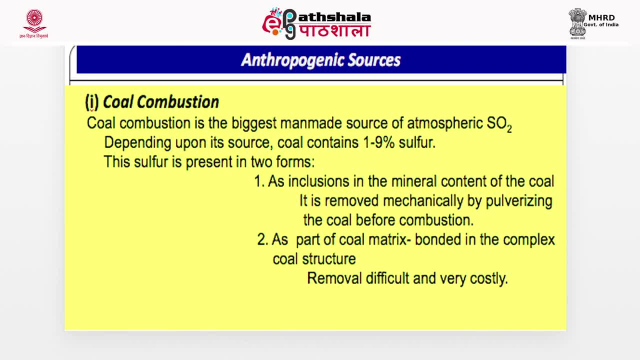 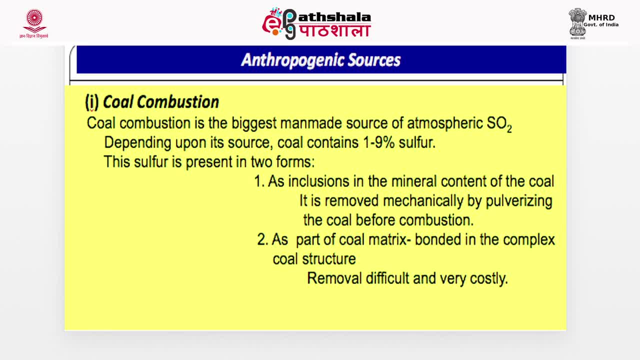 In fact As part of coal matrix bonded to the In the complex coal structure. If Sulphur is bonded to the carbons For Covalent bond made it That removal of such Sulphur is very difficult. 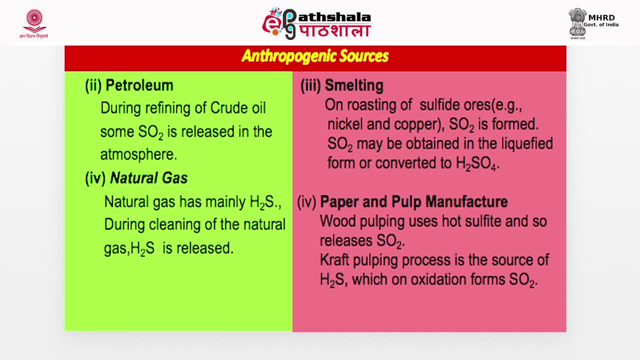 And costly So It cannot be done. Petroleum: During refining of crude oil Some SO2 is released in the At most. For example, At Muthra refinery There is gas That Despite their best effort To control SO2aintsion. 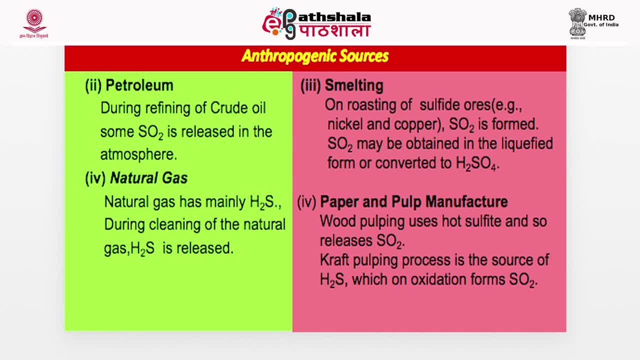 Some So2is released: Smelting And the roasting of sulphides For私. For example, decay and copper sulphides- SO2 is released. Now this actually what happens. The industries are running for business, for earning money and producing goods at cheaper cost. 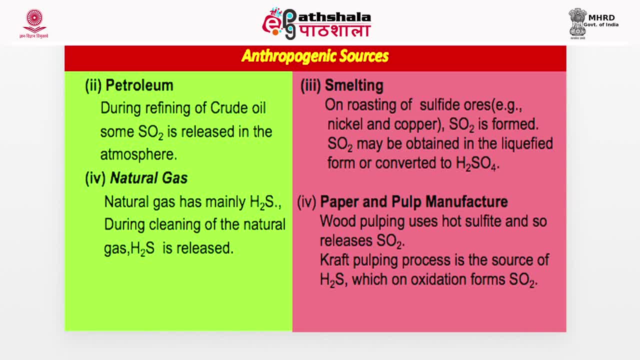 So if the amount of sulphur dioxide is large or sufficient, then this sulphur dioxide is used to form H2SO4 or sometimes to get sulphur element, elemental sulphur Natural gas. natural gas is mainly H2S, The CHG compressed natural gas that has methane. 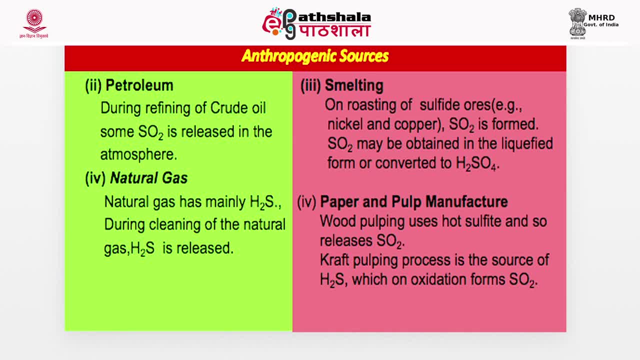 But it has some H2SO4, very small amount of H2SO4. This H2SO4 is cleaned before CHG is supplied. Paper and pulp manufacture: When the paper is made wood pulping, it needs sulphite Na2SO3. 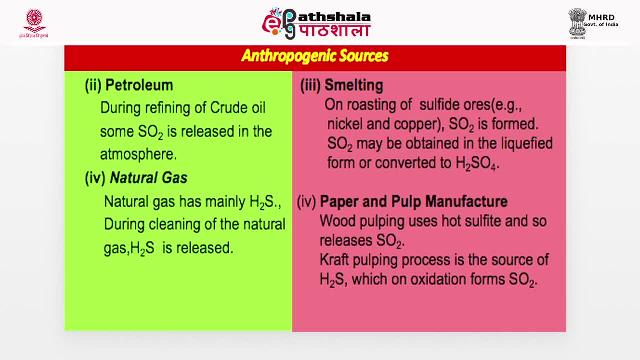 Okay, this is used there. This chemical is used in wood pulping And therefore it is a source of sulphur dioxide in the atmosphere. NOx, Remember this. NOx combines two compounds, NO and NO2.. But remember NOx and NO2O. 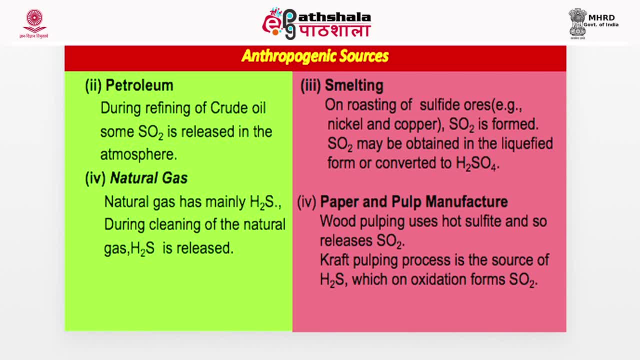 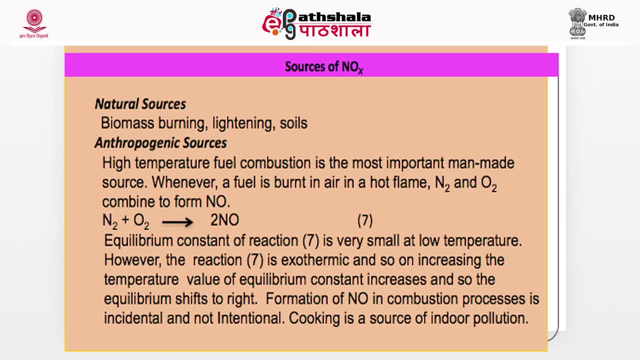 NOx means only NO, nitrous oxide, nitric oxide and NO2, nitrogen dioxide. Natural sources of NOx are biomass burning, lightening, and soils- Soil by aerobic biodegradation, NOx are produced. Biomass burning whenever you. 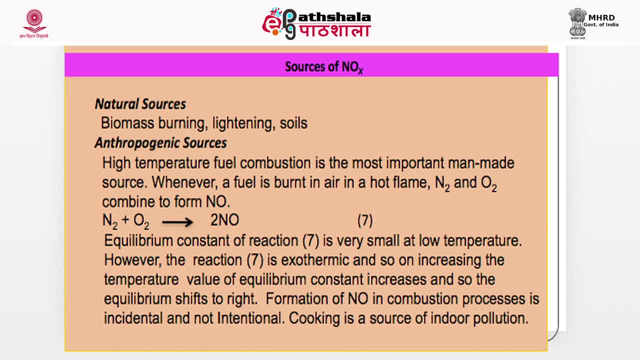 Nox Whenever any wood undergoes combustion at the temperature that is produced. at that temperature, nitrogen and oxygen combine to form NOx. That is, biomass, burning, Lightening. I already explained Anthropogenic sources, high temperature sources, Whether it is a kitchen, whether it is a fuel. 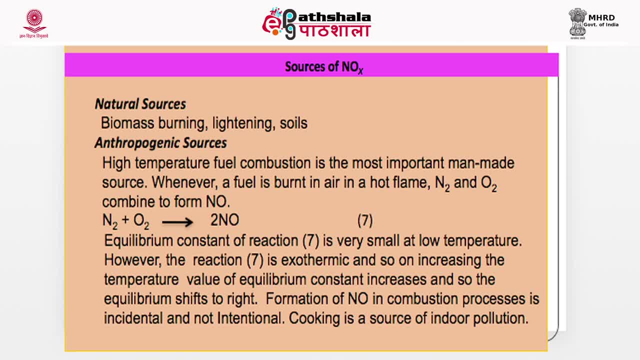 whether anything which occurs at high temperature, nitrogen or air is there That nitrogen and oxygen, they react to form NOx. This is a equilibrium reaction. This equilibrium is very small at low temperature, But as the temperature increases, the value of the equilibrium constant increases. 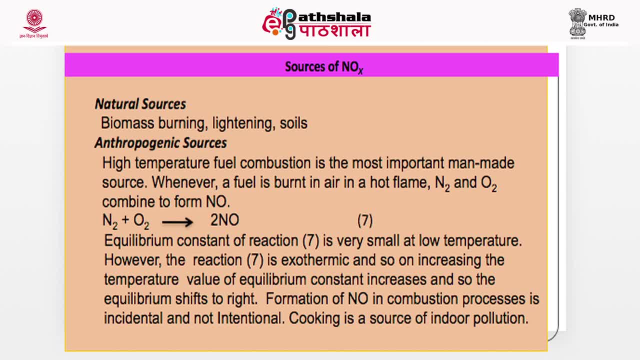 and this reaction shifts to right. So at high temperature more of NO is formed. So NO is formed from NO2 and NO2O reaction only at high temperature, Not at room temperature. At room temperature virtually there is no reaction. What would have happened if there had been a reaction between NO2 and room temperature? 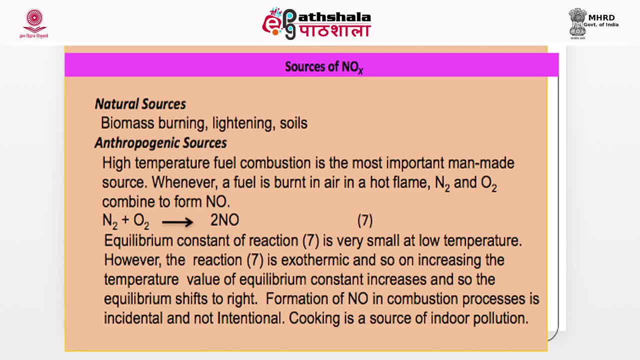 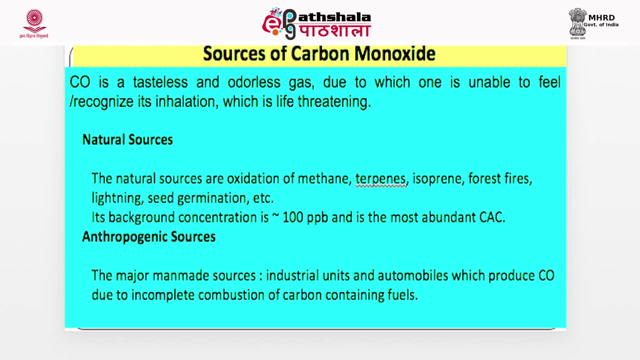 There would have been no oxygen and there would have been no life on the earth. Carbon, NOx- it is a criteria here- pollutant. It is a very dangerous substance. It is tasteless and odorless, Due to which one is unable to feel. 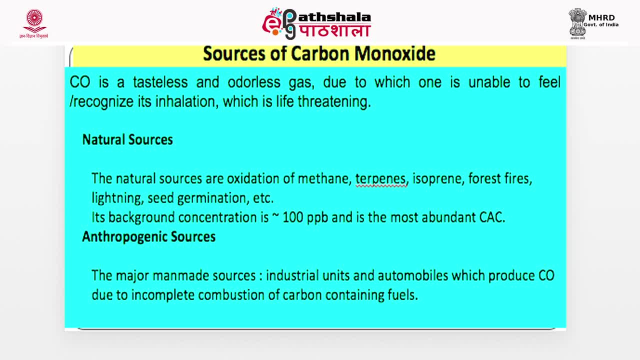 recognize its relation, which is life threatening. What happens If, in a closed room, particularly in winter, you sleep and you allow cold water to heat up the room? if there is not sufficient ventilation, slowly and slowly, the oxygen in the room will be. 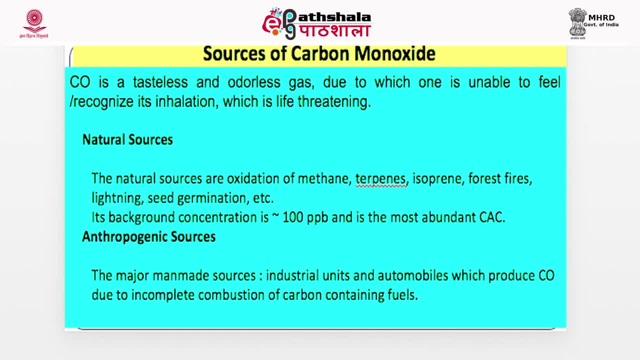 used up, oxygen will decrease and the combustion will form CO. The beauty or dangerous thing about CO is you get some kind of by inhaling some kind of nausea, So you don't feel it, you enjoy it, And this enjoyment costs life. 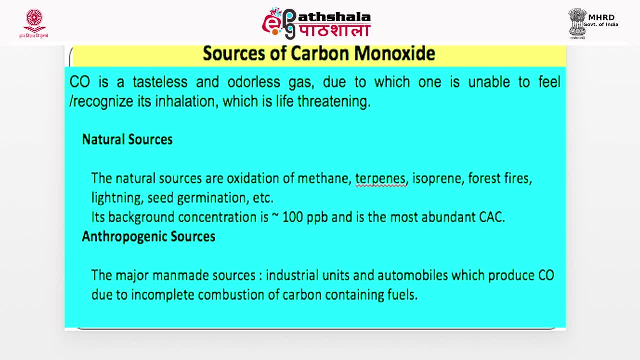 Natural sources of carbon, NOx. the natural sources are: oxidation of methane, terpenes: terpenes are released by plants, isoprene, again released by plants. Remember there are many organic compounds and inorganic compounds which are released by plants. 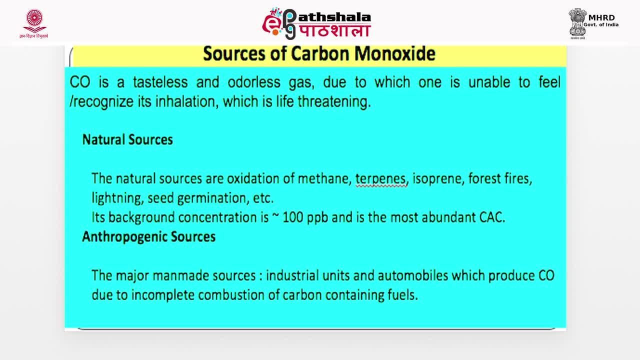 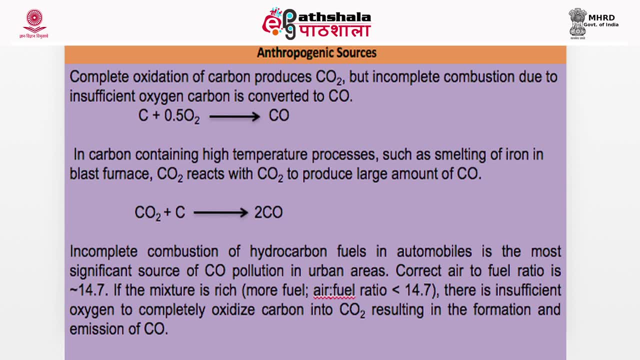 in their natural activities: Forest fires, lightening, seed germination, etc. They are natural sources. The background concentration of is 100 ppb And it is the most evident criteria. air contaminant Manmade sources are industrial units. 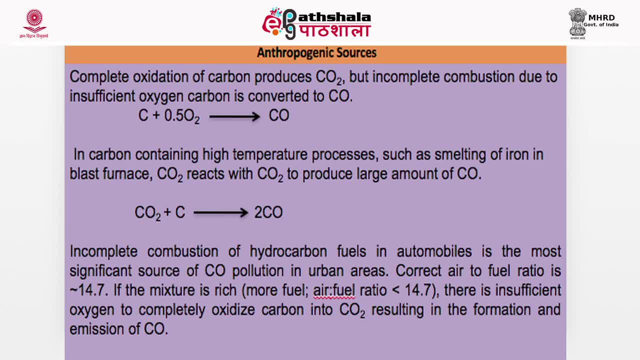 Manmade sources are high temperature sources, otherwise industrial units Due to incomplete combustion of fuel. Remember, carbon should be completely oxidized to CO2 by your C plus O to CO2.. What happens? Somehow the reaction occurs: C plus O. 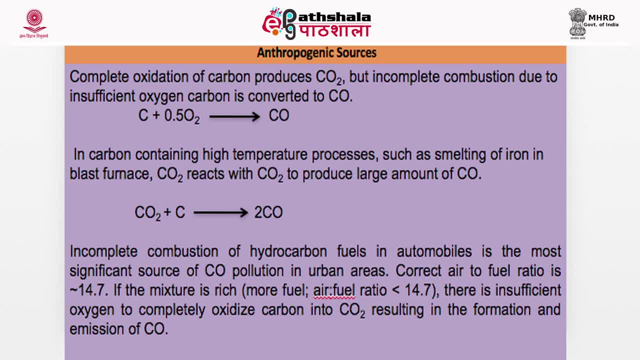 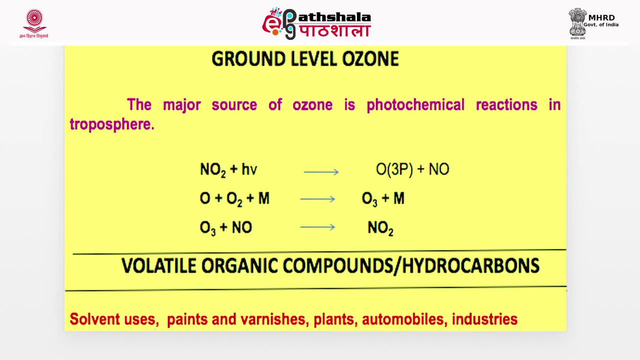 twice C plus O twice CO. The CO is not further oxidized to CO2 completely. Then what happens? Part of carbon is oxidized to CO and part is oxidized to CO2.. Oxygen, this ozone, Ozone, is an interesting gas. 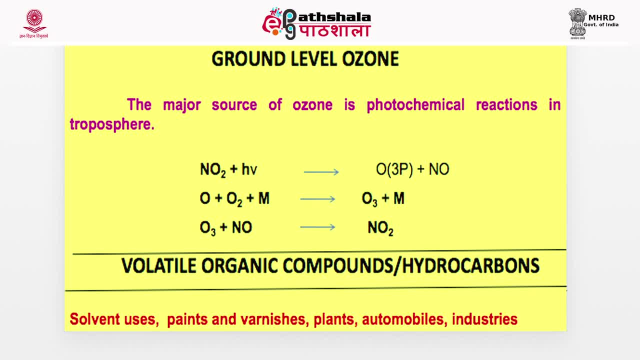 It has both roles. It is saviour of life, It is necessary in the status we have. But in troposphere, in ground level, ozone is a pollutant, It is a toxic material. So same substance can behave in both ways. 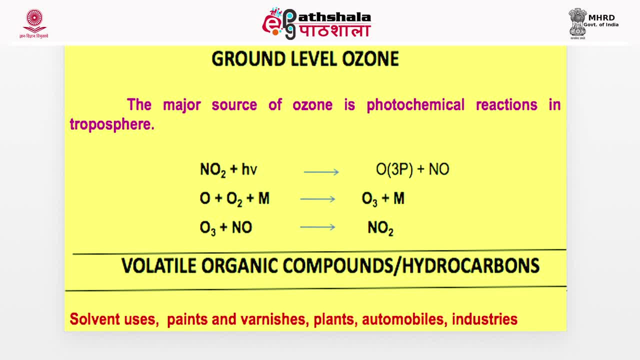 The classic example is ozone. How it is formed, The photo and nitrogen oxide which is present in atmosphere. by visible radiation of 390, 390 nanometer, It dissociates, gives you oxygen. This is ground state oxygen atom. Ground state oxygen atom and NO. 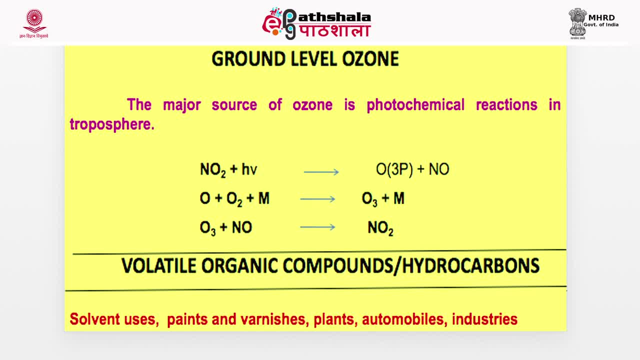 This O reacts with O2 to form O3. This M is a third body. The purpose of this third body is to remove extra heat that is removed, Energy that is removed. If it is not removed, then this will form the axial state and reconvert to it. 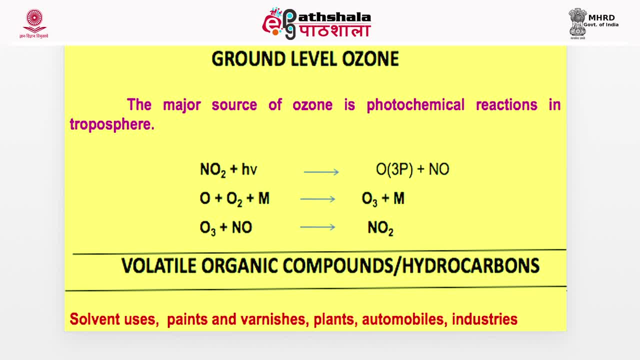 Ozone reacts with NO to form NO2.. So this is a three step cycle. NO2 was used up and regenerated And in this cycle ozone is formed. Volatile organic compounds: Another pollutant. The uses are solvents, plants and varnishes. 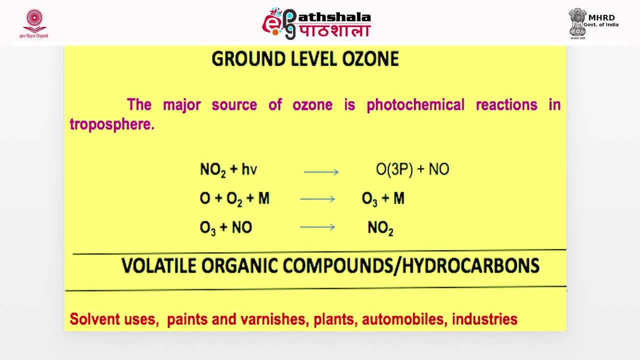 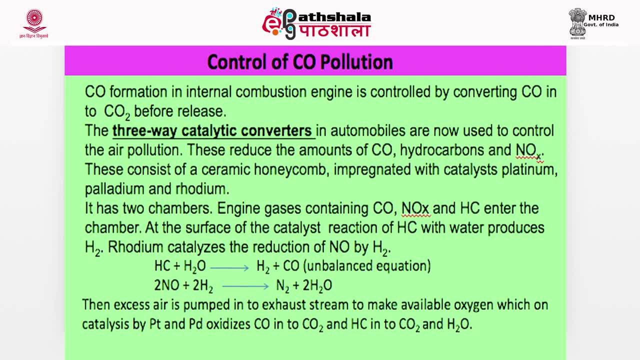 plants, automobiles and industries. Control of CO pollution, How it can be controlled. CO formation in internal combustion engine is controlled. How it is controlled It is. this is Three way. catalytic conversion- All the vacancies in India Now they are mandated to use catalytic converter. 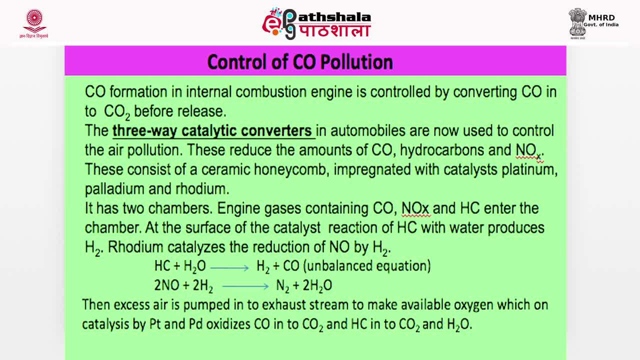 Use catalytic converters. They are factory, The factories, They are. All factories are required to. This catalytic converter must be in any car that is sold out. Now, what it does? It does so many things. It oxidizes CO2, carbon dioxide. 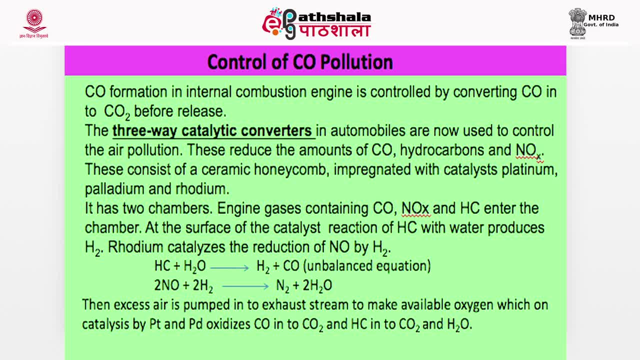 So no carbon monoxide is released in the atmosphere. Hydrocarbon, that is diesel or petrol. It is oxidized to CO2.. And NOx, that is formed because of high temperature. It is reduced to N2 and O2.. So it is done to check the release of carbon monoxide. 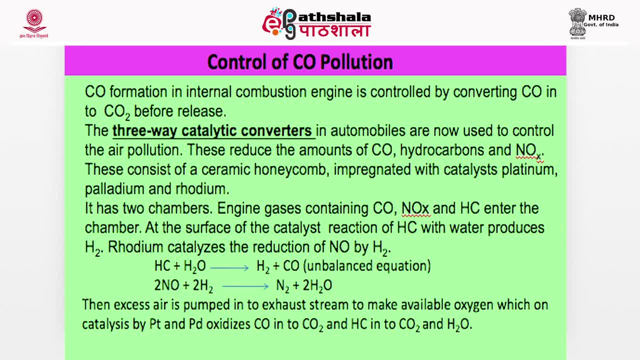 Hydrocarbon, said NOx Chemistry. The catalytic converter is a ceramic honeycomb type thing. It is impregnated with catalyst Platinum, palladium and rhodium- Remember they are caustic metals. They are used in it, So that is why it has. 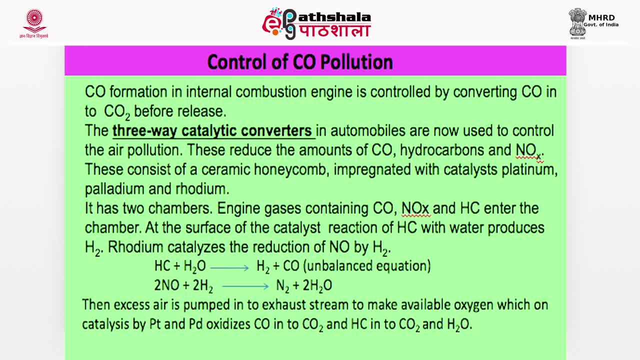 It is a catalytic converter that is used in cars. It is a costly material. It has two chambers. Engine Gases convert Containing CO, NOx and SC enter the chamber And the surface of the catalyst reaction of SC with water produces hydrogen. 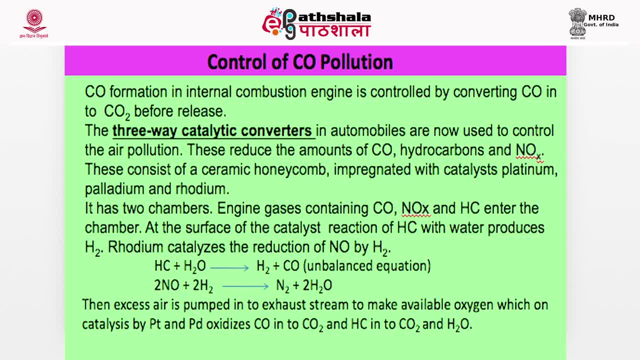 This reaction And this hydrogen reduces NO2, N2.. So this, What has happened? Hydrocarbon as well as NO, Both have been removed In the second stage. Then excess here is produced, Then excess here is pumped into the exhaust stream. 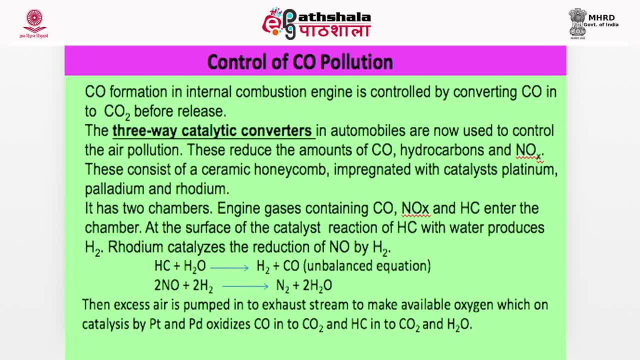 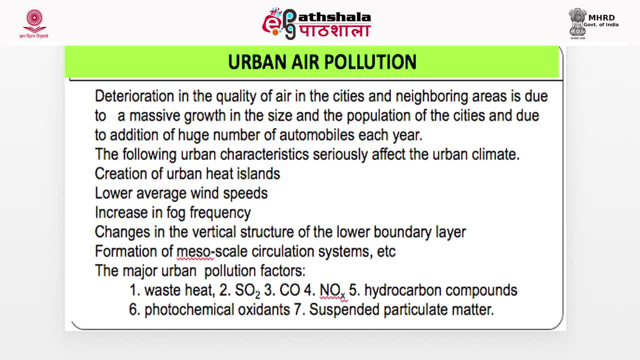 To make available oxygen, Which are catalysts. These catalysts, CO is CO2. And SC into CO2 and water. So this is how catalytic converter works. Urban air pollution. Now we know the cities and villages, Rural areas. 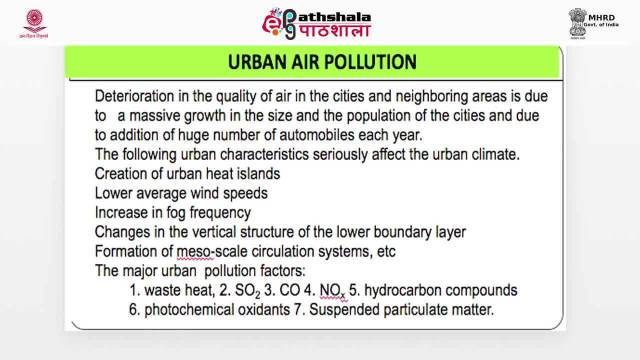 Which are more polluted. The cities are more polluted Than the rural areas. Why? Because of massive growth In the size and population of the cities, Addition of huge number of automobiles each year And what happens, Falling urban characteristics seriously affect the urban climate. 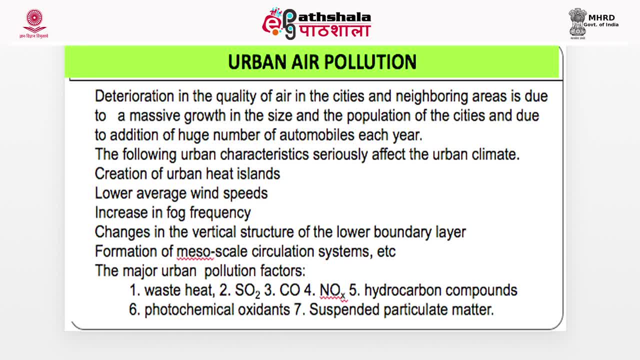 These are the. They are typical, Peculiar to cities only: Creation of urban heat islands- I will explain later on. Lower average wind speeds, Increasing fog frequency, Changing the vertical structure of the lower boundary layer, Formation of mesoscale circulation systems, etc. 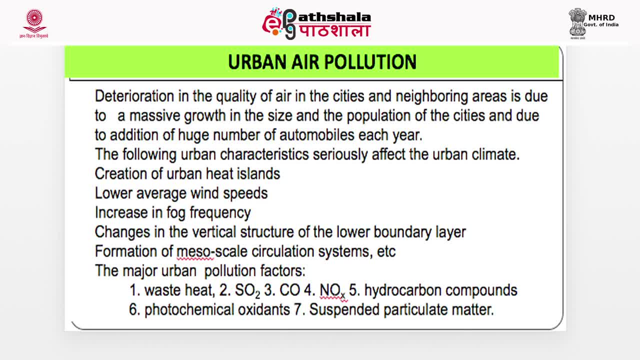 These are the some major things which happen In cities. The major urban air pollutants are Waste heat, Sulphur dioxide, CO, NO2.. Hydrocarbon compounds, Photochemical oxidants, Suspended particulate matter. How come The waste heat is very important thing. 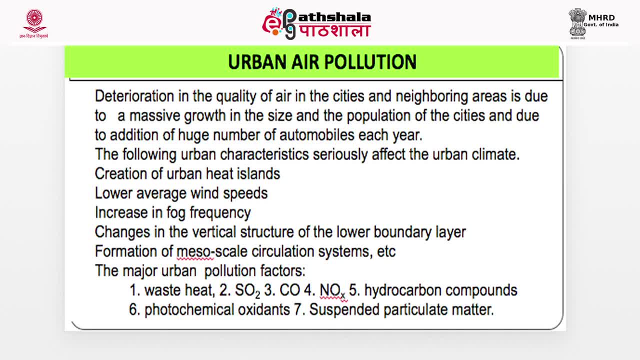 In cities There are large number of air conditioners, Almost 30% homes or 25% homes They have air conditioner. Part of is, If your room is cool, Where the heat has gone. The first law of thermodynamics says: 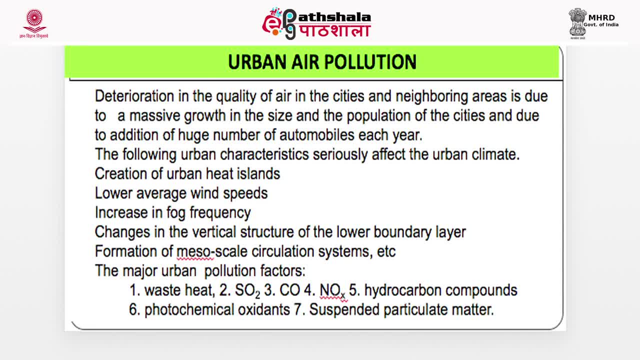 That heat, The energy cannot be Created, nor can be destroyed. So the energy, you have not destroyed It, you have simply released outside. So it is in the outside That heat is outside. Another thing: The walls and the houses. They are made of concrete. 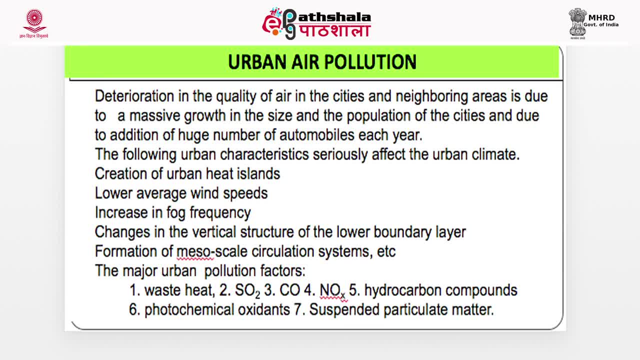 Stone Or cement. During day time They become very hot, They absorb Energy And store it, And after it They start releasing this heat. So each of the, Each of the building Becomes a source of Heat. 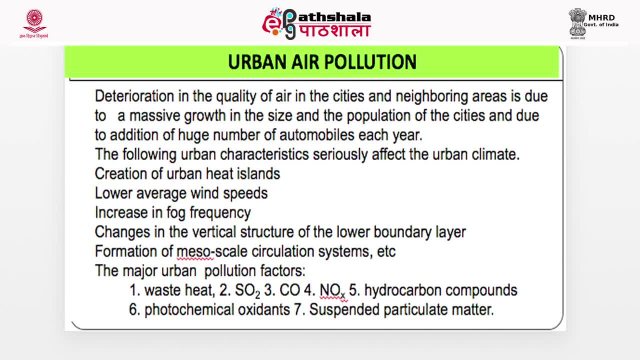 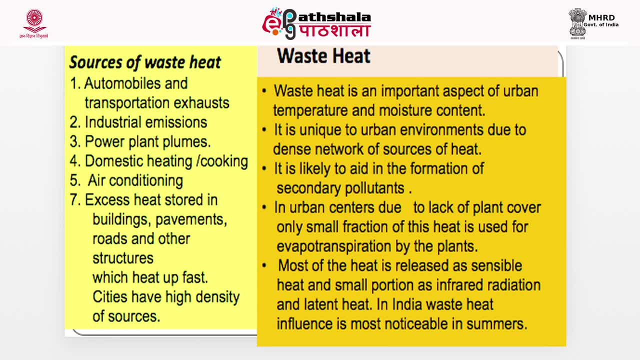 So that is how waste heat is Reduced, Released in the atmosphere. These are the sources of waste heat: Automobiles and transportation Exhaust. You know How hot is the Exhaust of the car Or motorcycle If you touch it. 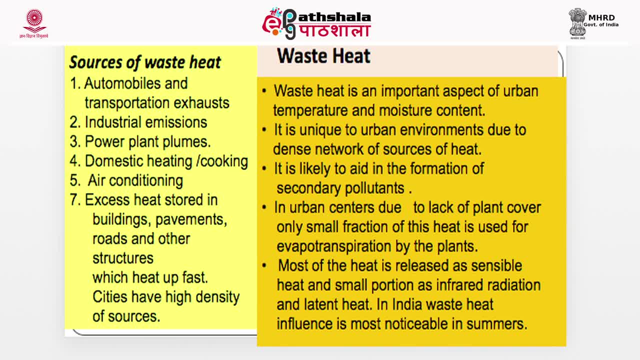 Your skin will go off. It is so hot. Industrial emissions- Power plant plumes, The smoke coming out of the power plant. It is also very hot: Domestic heating and cooking, Air conditioning. Excess heat is stored in the buildings. 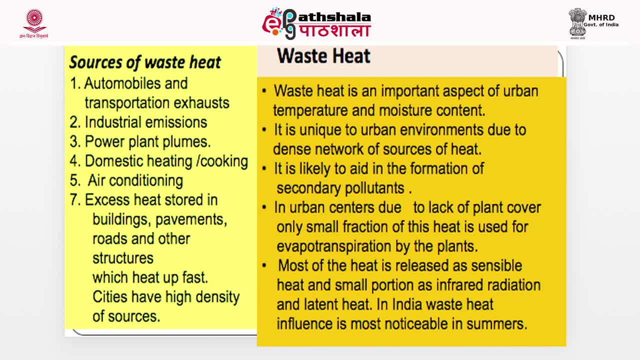 Pavements, Roads. You move in the summer, I mean In the next month. If you You move Barefoot On the road, You will have Trouble Moving Waste. heat is an important aspect of urban temperature and moisture content. 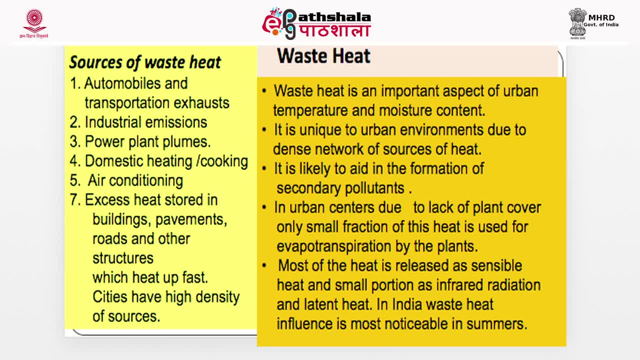 It is unique to urban environment due to dense network of sources of heat. Every house has a kitchen, Every house has a air conditioner Or some other source of heat. It is likely to end the formation of secondary pollutants In urban centers due to lack of plant cover. 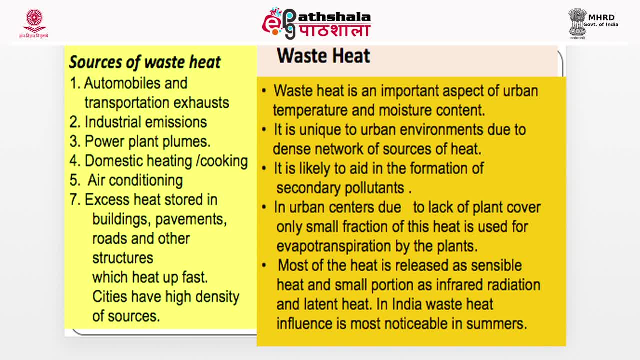 There The number of plants is very small. Most of the heat is released as sensitive heat And small, Small portion as infrared radiation And latent heat. In India, Waste heat Influences, the most noticeable in summers. We all know it. 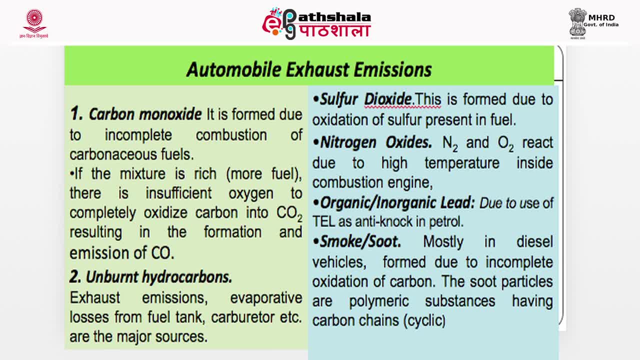 Auto oil exhaust emissions, The vacuums, What they release: Carbon peroxide Due to incomplete combustion, Unwanted hydrocarbons And And, And, And, And And. divorces from the exhaust of your vacuums. 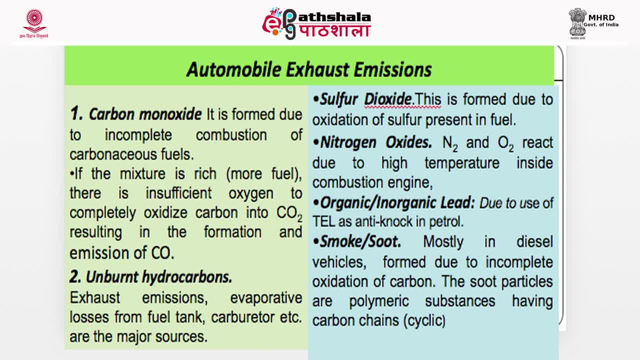 Evaporative losses from fuel tanks And Carbohydrates, Etc. It will be interesting for you to know that If you put your vacuums outside for some days And you put a 5-liter petrol tank And after 10 days you will find that the petrol tank is not 5 liters. 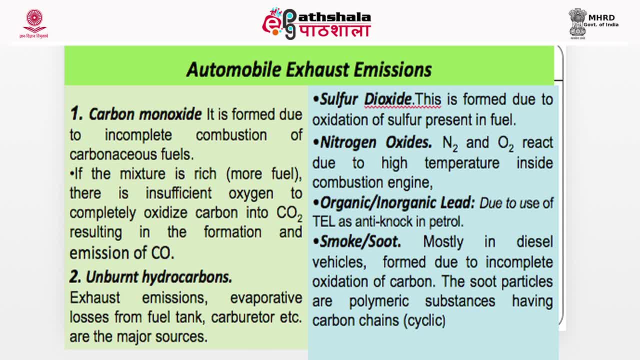 What happened to it? It evaporated. What will happen when you control the defecation But an evaporative loses become less And the Beer Da-Weis 211. lt. and this: It evaporates If your tank is full. so if you keep your tank of your vehicle full of the fuel, then the losses due to emission losses from evaporation are less. 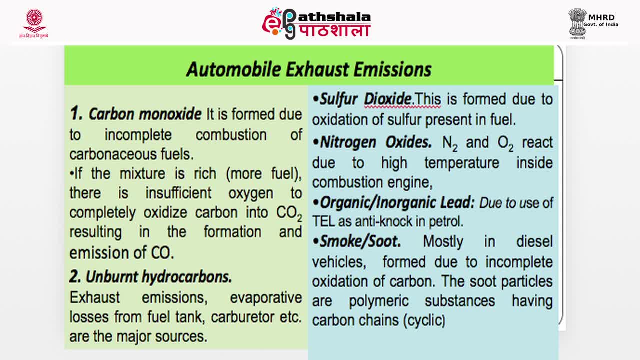 Sulphur dioxide, but in fuels the sulphur dioxide is not much, but this is important Because at high temperature nitrogen-oxygen compound is combined to form NOx, organic-inorganic layer. Earlier antinox compound was used to increase its octane rating efficiency of the petrol engine. 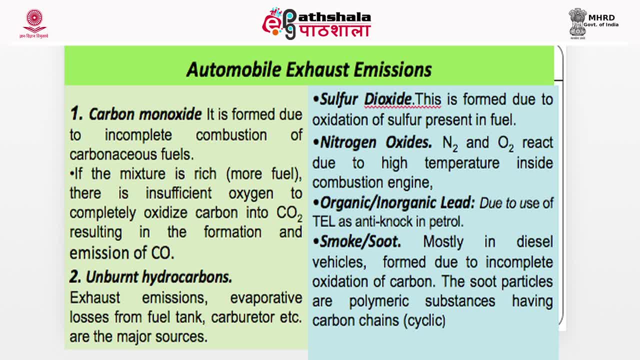 But in most of the countries this has not been used. Smoke chute is mostly diesel type vehicles. You see the smoke coming out of a diesel vehicle or truck. you will find it is black. These chute particles: they are polymeric substances. 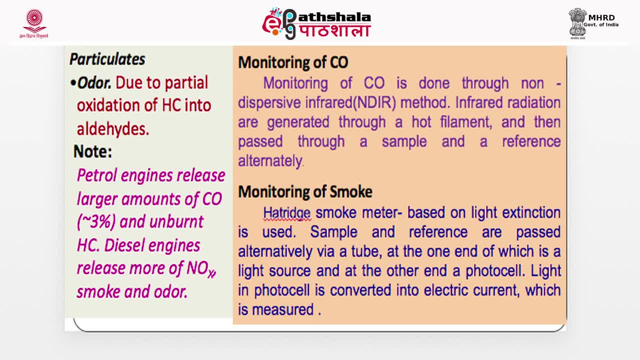 having carbon chains, particulates and an order due to partial oxidation of hydrocarbons into aldehydes, Particularly in the cities, For example in Delhi. here your eyes will have a burning sensation in winter In a city center where there is high traffic because this is due to the oxidation of hydrocarbons into aldehydes. 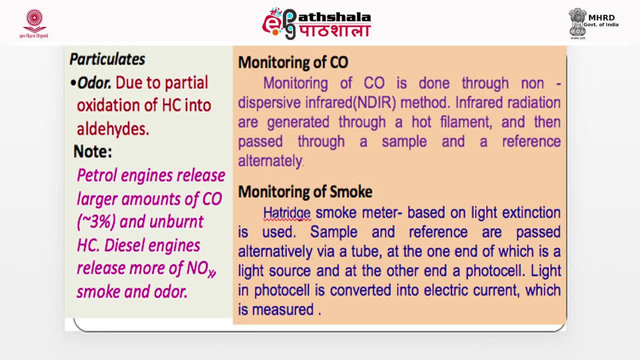 So this irritation- eye irritation- is due to aldehydes. Petrol engines release a larger amount of CO. Diesel engines release more of NOx, smoke and aldehydes. So that is the difference between these two How CO is monitored. 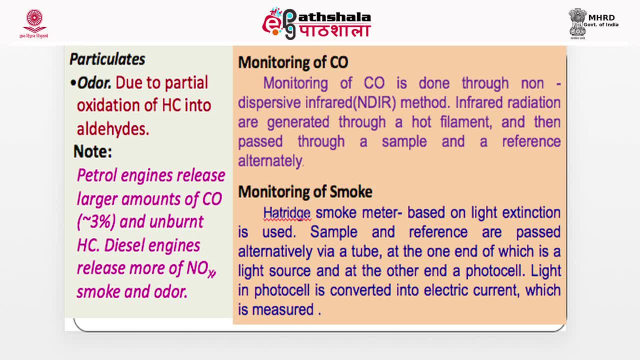 CO is this tank? this is the name of the technique. details are not given. Non-dispersive infrared method is used: Smoke. for measuring of the smoke, Heart rate is used. Now how we can control the pollution by our vehicles. 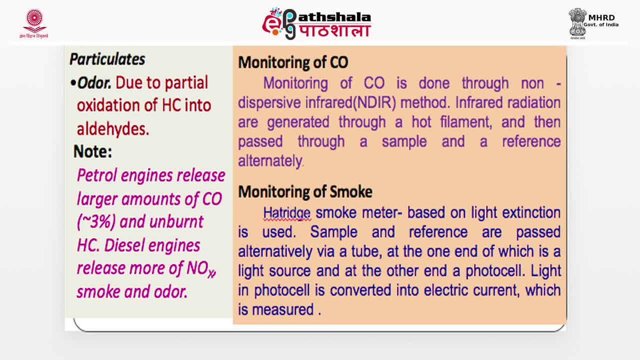 The proper maintenance of the engine. This will increase the life of the engine. Better efficiency, better mileage. The petrol tanks should be full Use of kinetic converters. it is not necessary. It is necessary everywhere now, Regional and global pollution. Pollutants released at one location are known to be transported over large distances, and sometimes without much dilution, from one country to another. 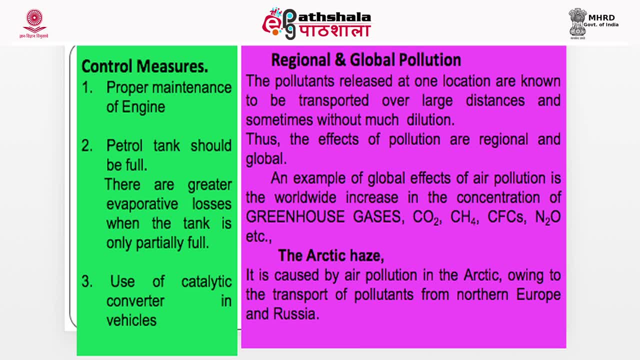 Thus the effects of pollution are regional and global. An example of global effect of air pollution: with worldwide release increases the concentration of greenhouse gases Because actually they have a long life. CO2 has a long life- 44 years. CO2 has a long life of 90 years. 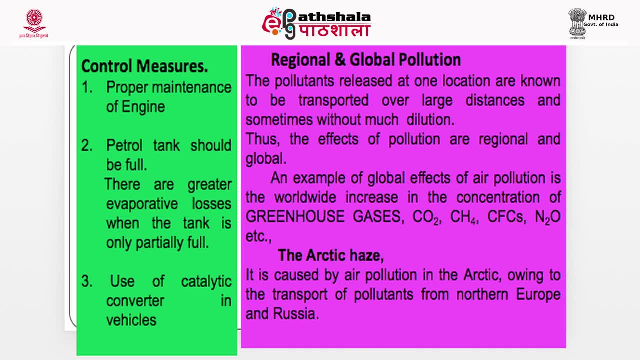 N2 has a life of 150 years, So during this the time is sufficient to move from India to USA. Arctic haze: it is caused by air pollution in the Arctic Pole, North Pole, Going to the transport, Going to the transport of pollutants from Northern Europe and Russia. 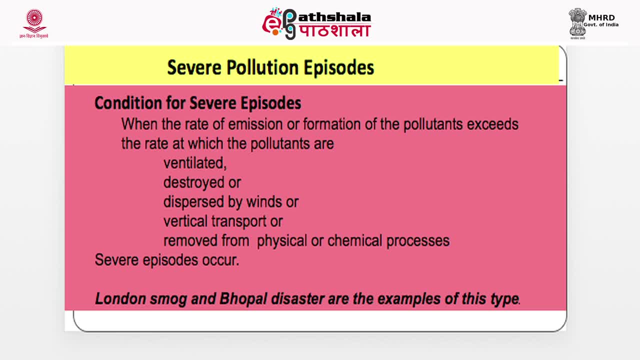 Severe pollution episodes. You must have heard Bhopal episode, London smoke. Remember the pollutants which are released in the atmosphere. They do not stay forever in the atmosphere. What happens? They are removed from the atmosphere. So there are two processes. 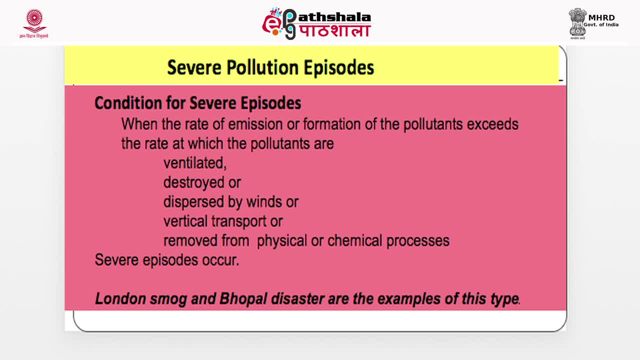 One: the rate of emission or formation of the pollutant Number. the rate of release or removal of the pollutants. If this is greater than this- There is more release than removal- Then what will happen? The pollution will increase. Pollutants are removed. 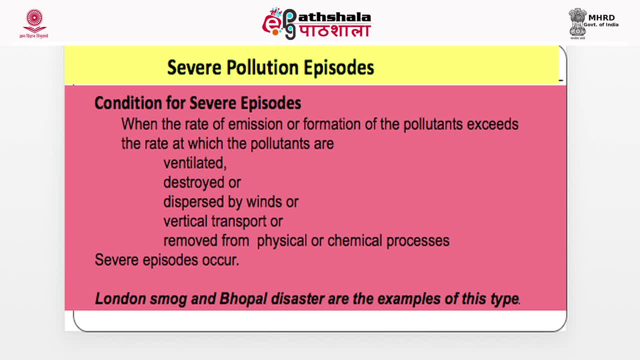 How? By ventilation, By destruction, By dispersion winds, By vertical transport or removed from physical or chemical process. What happened in Bhopal? That was 1st or 2nd December night. It was winter, The wind speed was very low.